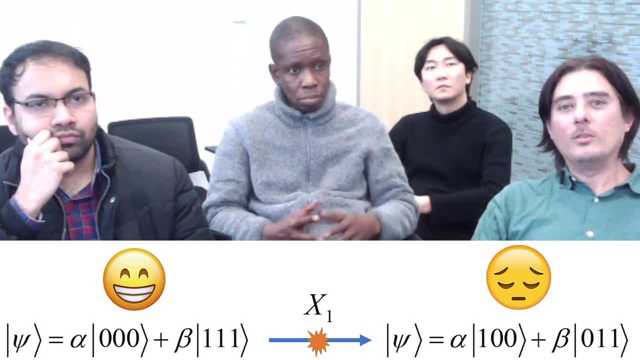 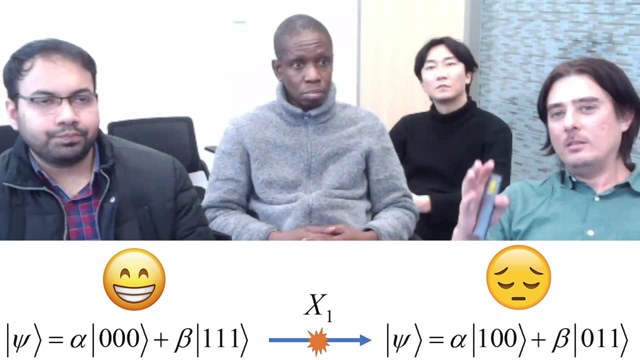 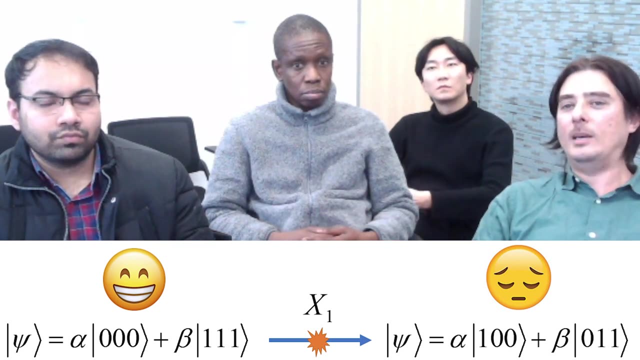 So if now an error happens, say on the first qubit, then as you can see, you can actually tell that an error has happened, Because obviously you know the odd man out here. for example, in the first one here, one zero, zero. you can tell that basically the error has happened on the first qubit. 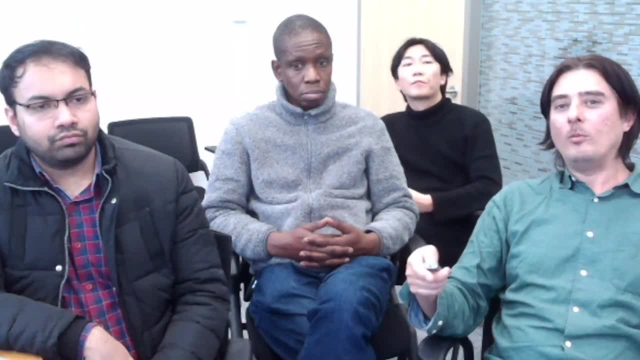 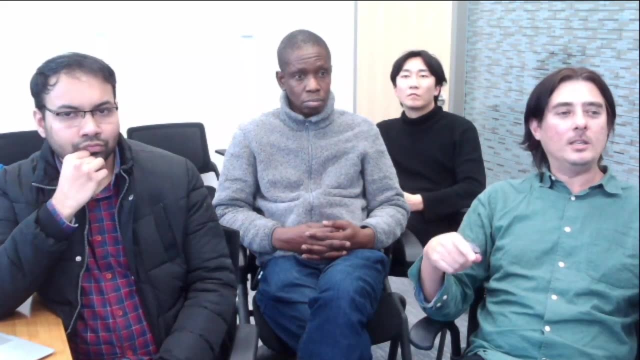 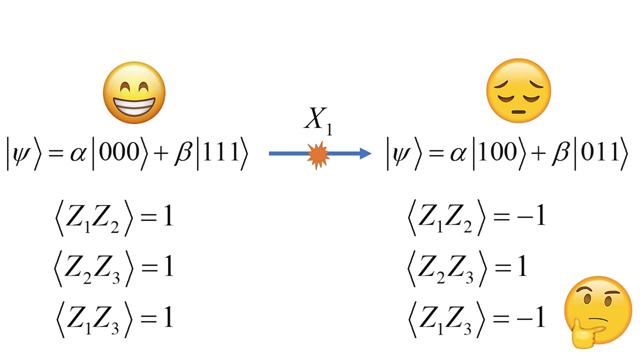 And that means that we can- We can- actually figure out what needs to be done to correct it. And the way that we actually figure out what qubit the error has happened on is using these so-called syndrome measurements, And in the case of the bit flip code, you measure these things observables like Z1, Z2, Z2, Z3, Z1, Z3.. 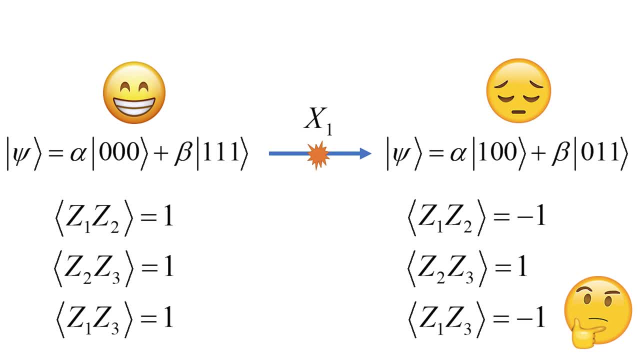 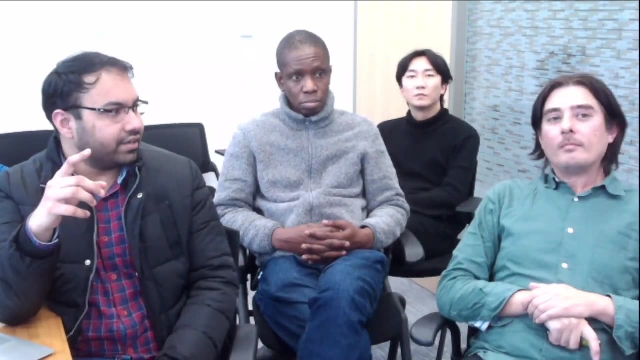 And if no error has happened, then these should all be basically one, But if an error has happened, then one or more of these flip, Then you can figure out where the error has happened. Is this a common way to duplicate the qubits and then check the error correction? 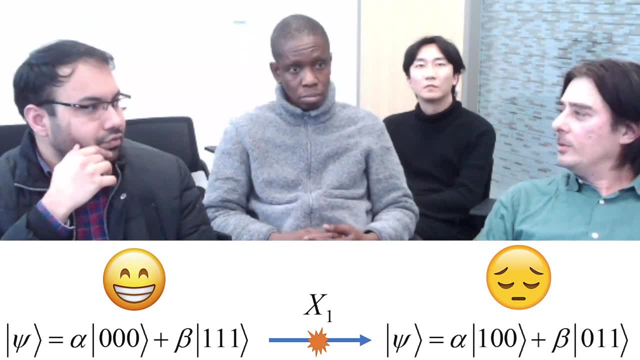 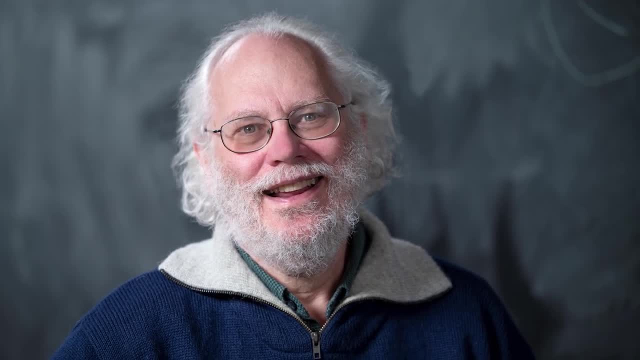 Right, yeah, So this is called the bit flip code, the one that I'm talking about right here, And this was basically one of the first error correcting codes. Actually, Peter Shaw was the one that actually, I think, thought of this. 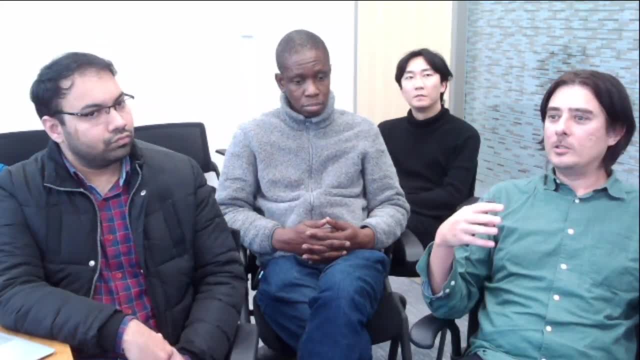 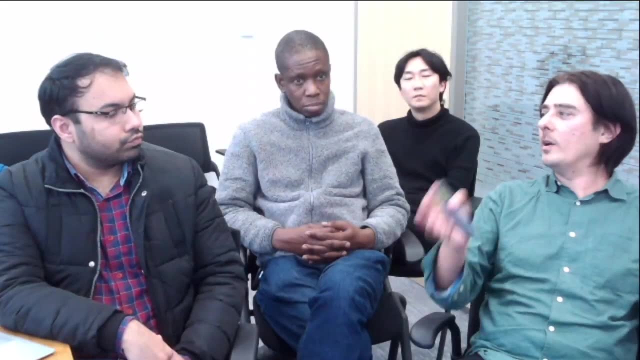 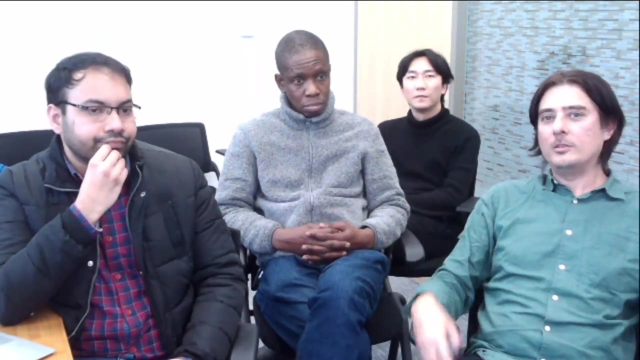 In fact he was the one that basically worked out the first nine qubit code. You're dead, You crazy son of a bitch. You're dead. So nine qubits making one logical qubit. And then people started to improve upon the whole kind of thing with various different tricks. 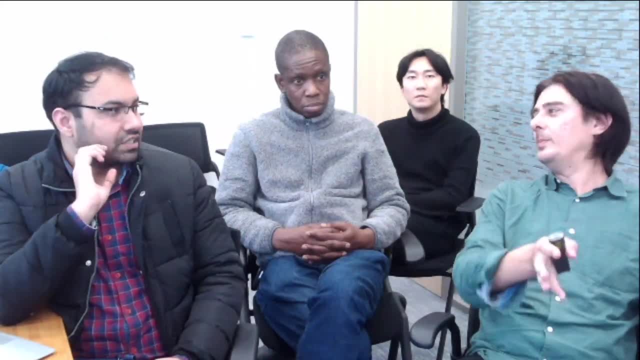 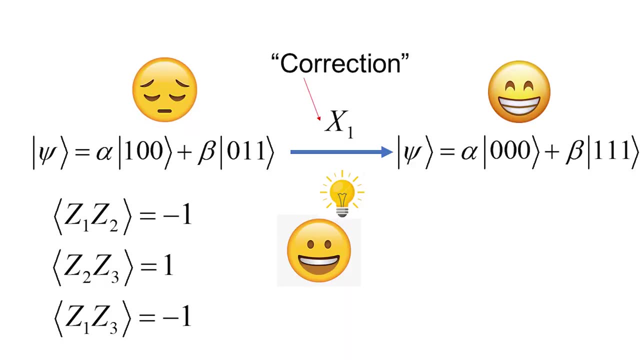 And these days there are much more modern codes, But conceptually this is basically what actually any error correcting code is always doing. So, going back to our example here, So if you figure out that the error has happened on like the first qubit, 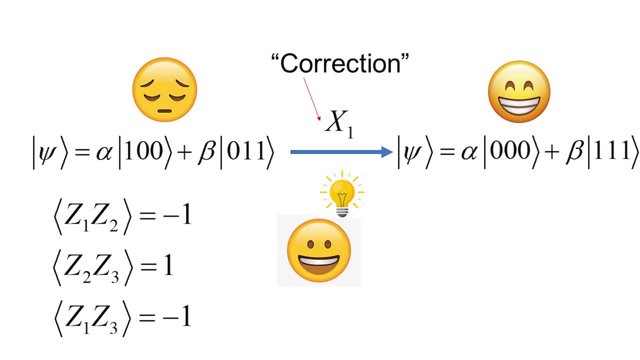 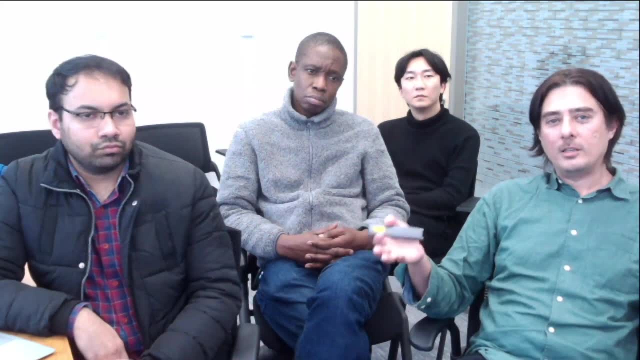 then basically all you have to do to correct it is to apply another X gate on the first qubit, and then you're back to where you started, And so this completes, like the quantum error correction cycle. So this is basically the kind of thing that we want to do. 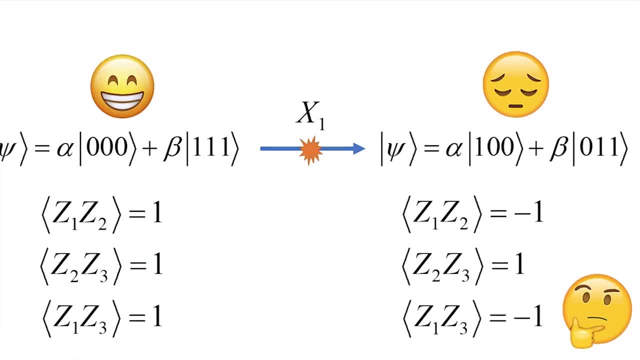 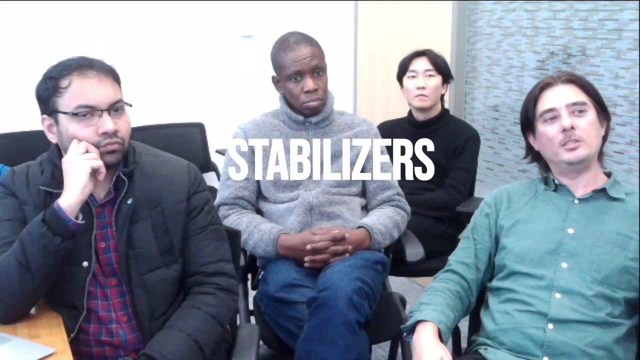 Now, the important thing here is that there are these operators that we just saw a few moments ago And these are called, in this context, stabilizers. right, And they're called stabilizers because the key property that these operators have is that you apply it to the states. 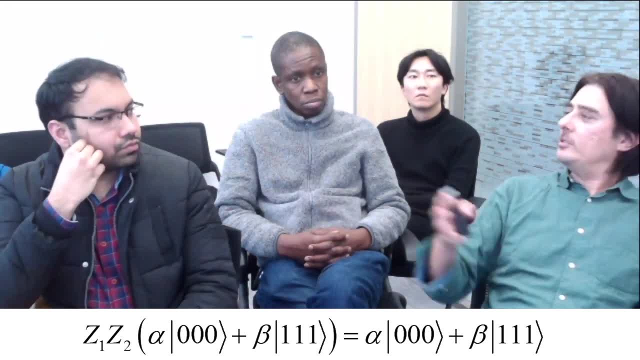 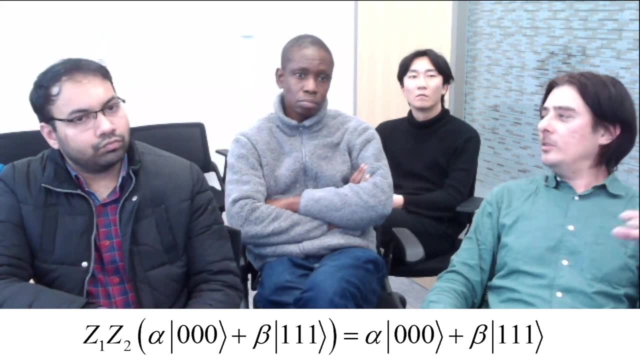 Yeah, And basically yeah, It doesn't change the state, right? So you can apply these measurements as many times as you want And basically it's not going to change the state. And so what you can do in this situation is that you know. 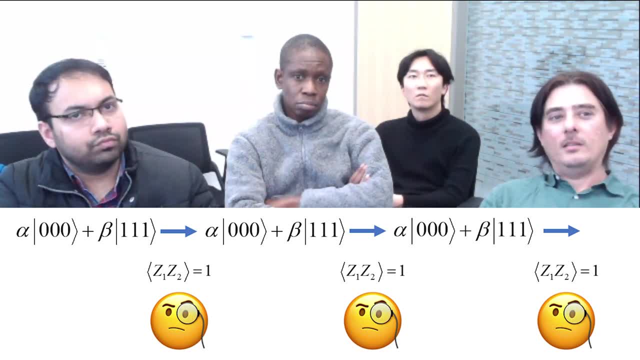 you can keep on checking whether the state has had an error on it or not, right? So you just go and say, okay, has an error happened. Okay, no good. Okay, an error happened. No good, No good. 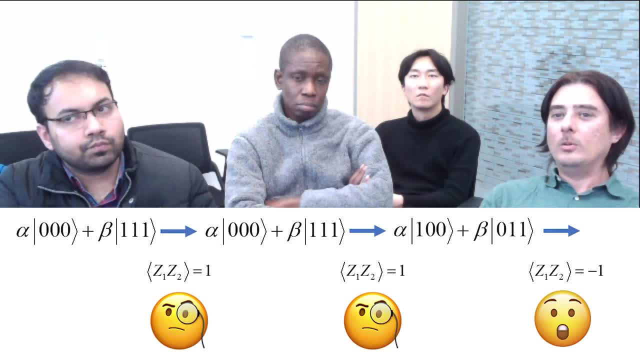 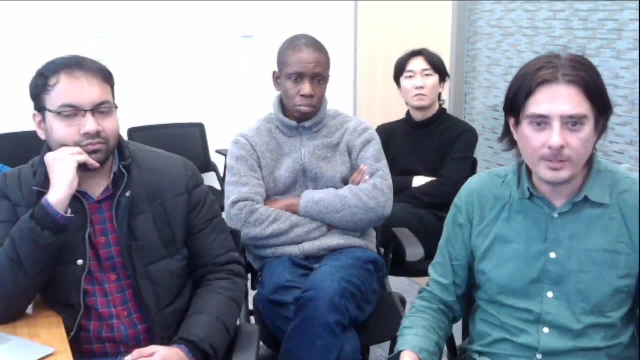 And then. but at some point an error will happen, And then you will realize: oh, an error just happened. Okay, now we can go and do something about it, right, Okay? so now let's go to basically what the Google paper has actually done. 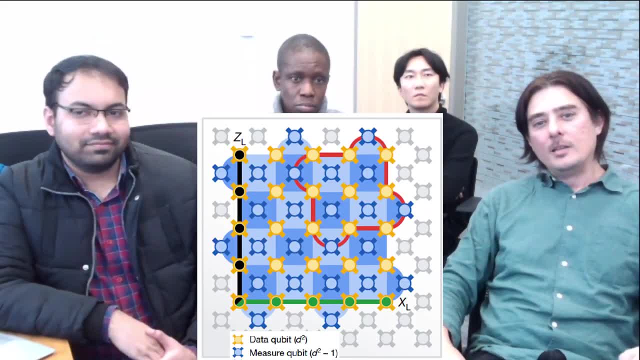 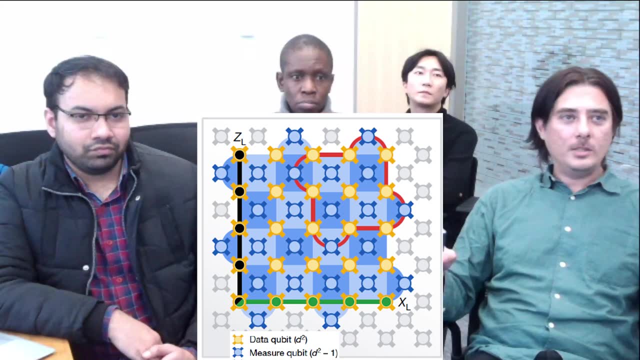 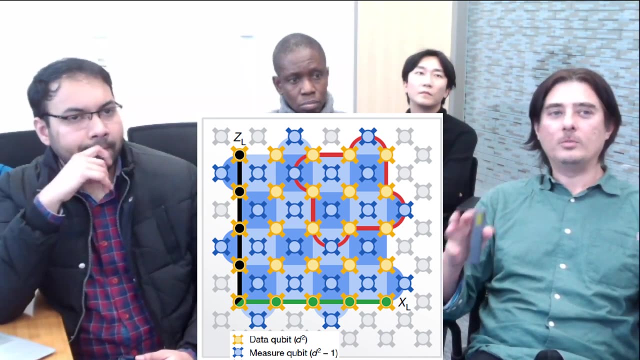 Okay, so this is like figure one in their paper. So what you see here is the arrangement of qubits, And so you have a bunch of yellow qubits here and a bunch of blue qubits. So let's first start off by looking at the yellow qubits, which is really the important qubits, which is storing the information. 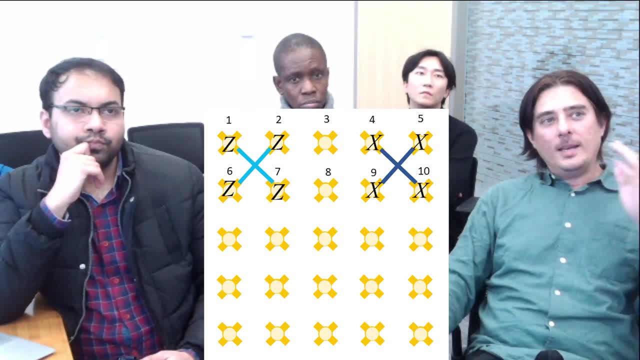 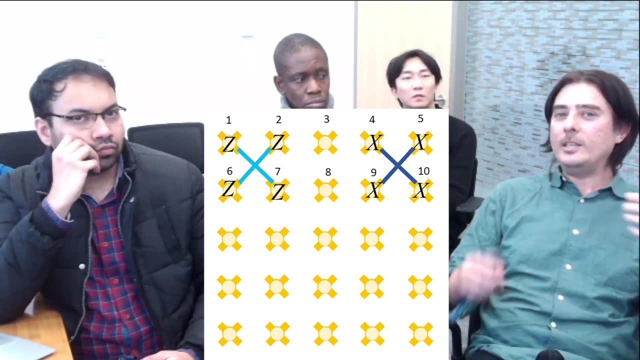 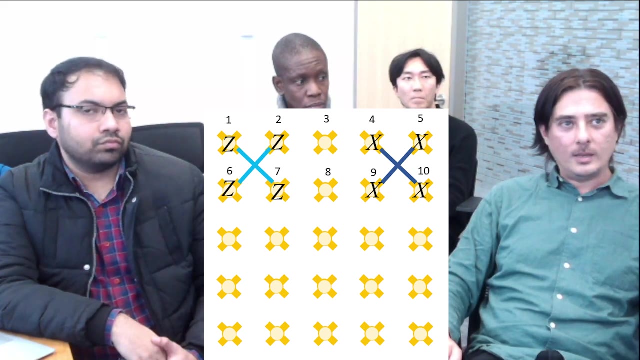 So, if you look at just the yellow qubits, what they use is a so-called surface code in order to basically encode a logical qubit. So eventually, this thing is actually just encoding like one qubit. The special property that these surface codes have is that you can apply these plaquettes. 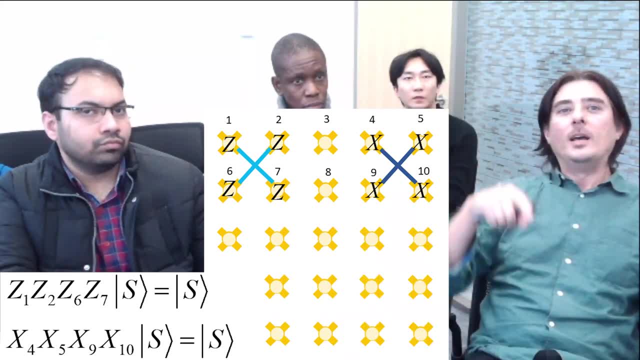 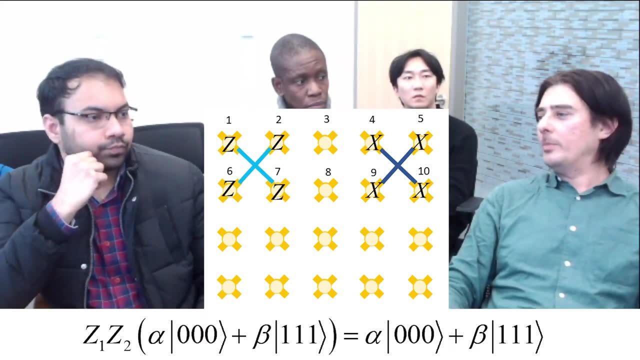 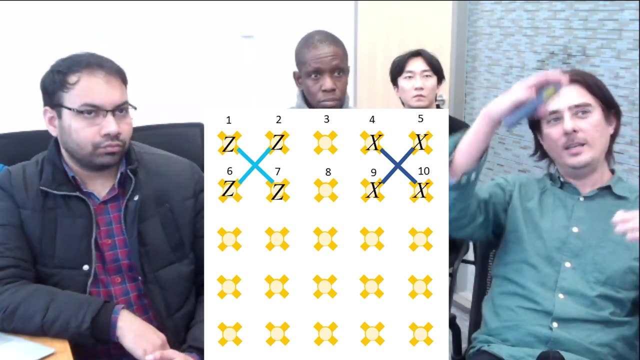 so these squares of operators to the state and state doesn't change. doesn't change, Just like the Z operators that I showed for that Simpler example before. In fact, the bit flip code that I showed is actually some limiting case of this surface code. 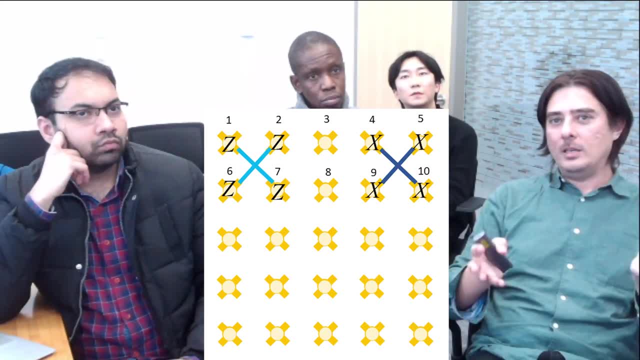 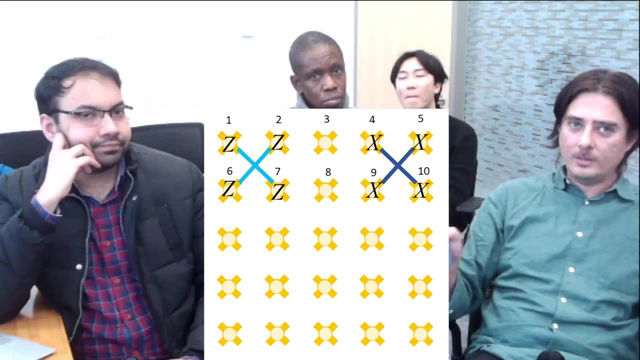 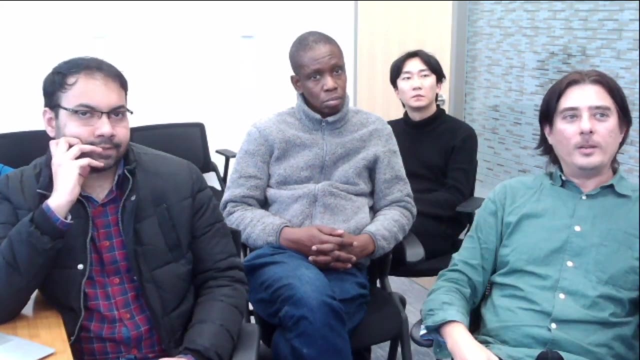 The difference to the bit flip code is that this thing can actually encode a full qubit, whereas actually the bit flip code can only correct for bit flips, And if there's a phase flip it doesn't work. But this one can fully correct all kinds of errors, at least for this one qubit. 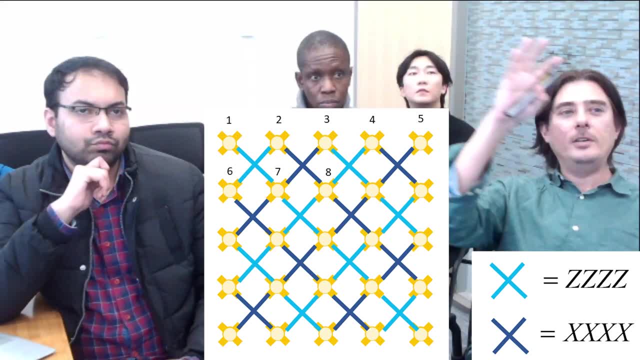 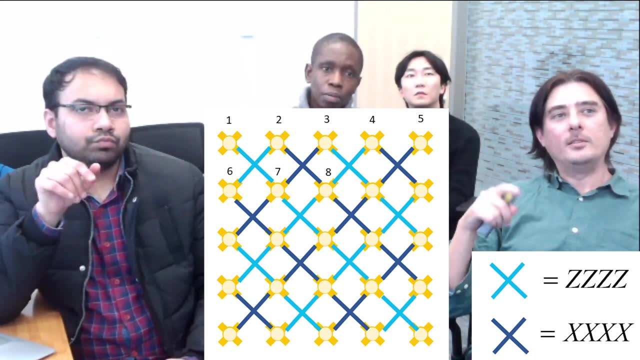 The Zs are oriented in this way, So it's sort of like every other plaquette is a Z Z square And then the alternating ones. the Xs are the dark blue ones here, And so they, if you apply Xs in those positions. 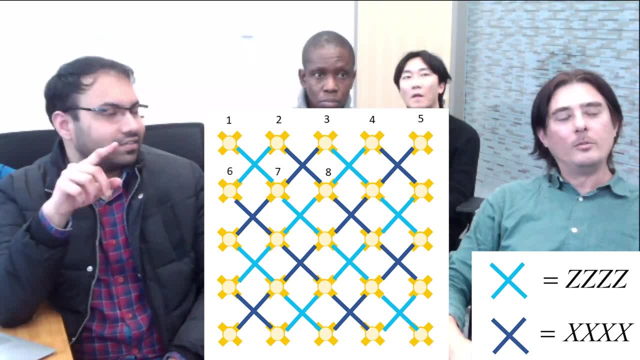 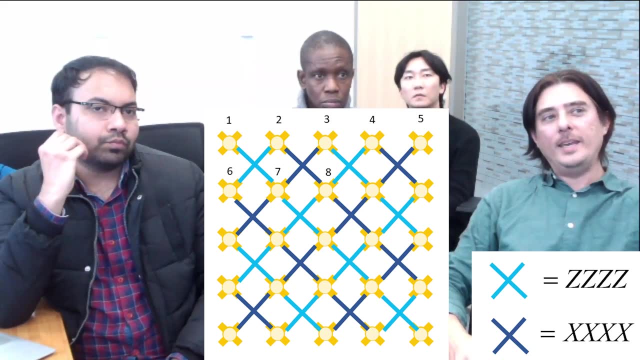 So no two Zs come together. I think, diagonally or Right, It's always four Zs actually. But there's one exception, which you might be thinking of, which is actually on the edges. There are actually some places where it's just two Zs. 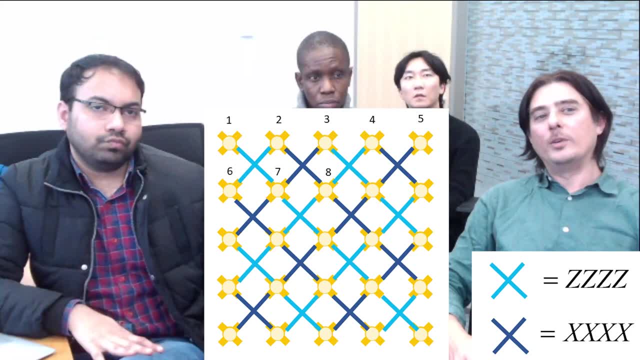 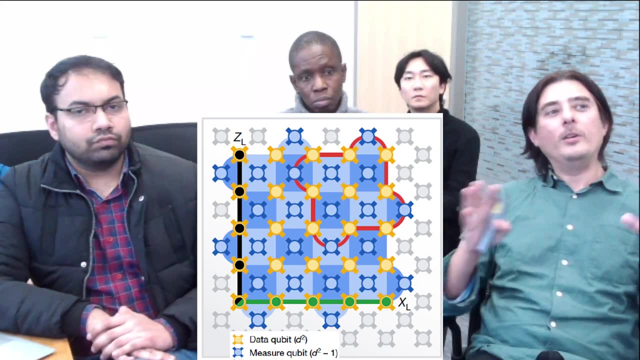 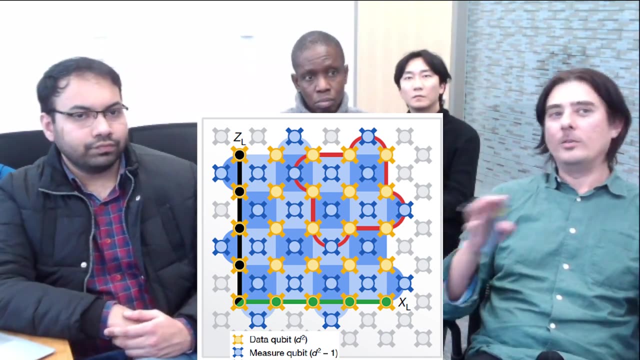 But generally, in the middle of the lattice, there's always four Zs or four Xs. That's basically the kind of state that we're making on the yellow qubits. So then, what are these blue qubits? Well, basically, in order to make that measurement of the four Zs or the four Xs. 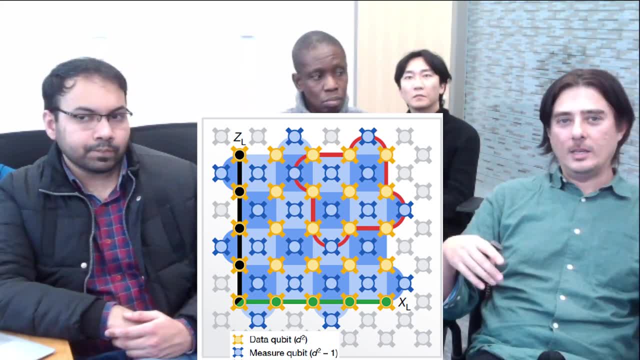 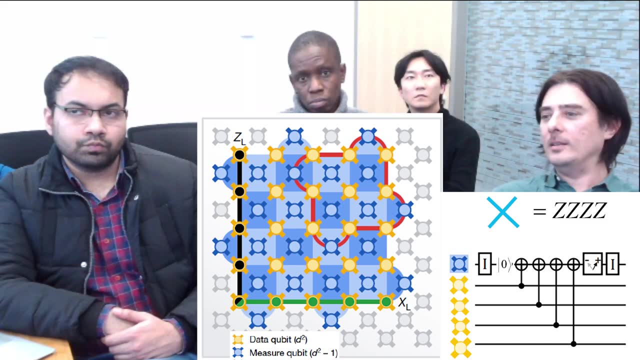 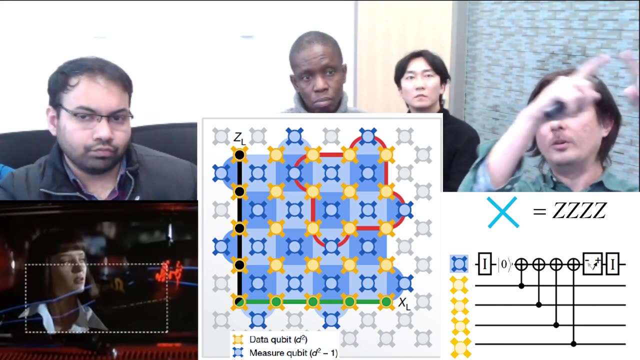 you basically need an ancilla qubit in order to do it. Basically, there's a little circuit that you can do, which is just on the right here, And the blue one is basically the ancilla or the extra qubit, And then the other four are the four real qubits arranged in a square. 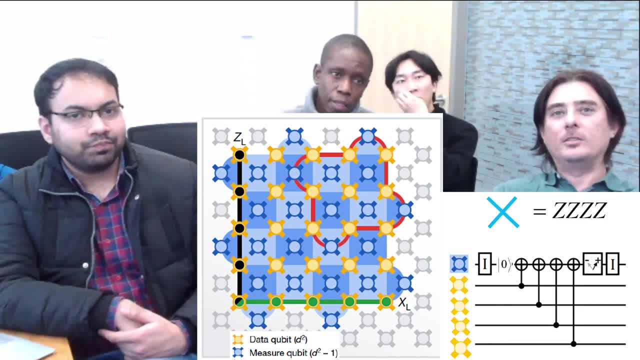 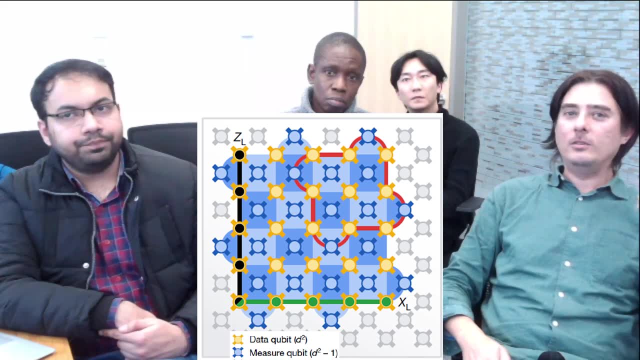 So you do that circuit there for all these different squares. Well, actually sorry, This one is for the four Zs, which is the light blue ones. For the four Xs, there's a slightly different circuit that you do, But the story is still basically the same. 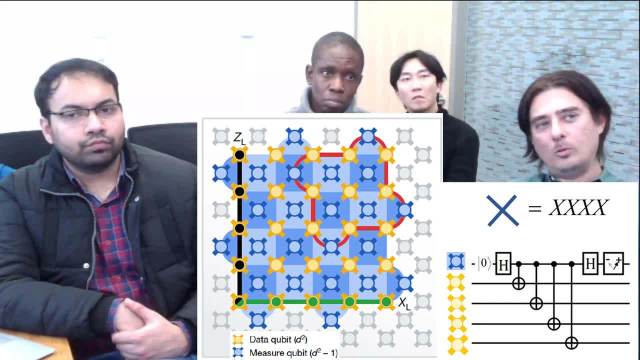 So in the middle of each square that you see in the yellow qubits, there's a qubit there which is purely performed there to do basically just the measurements of either the four Zs or the four Xs And the gray ones they don't use. 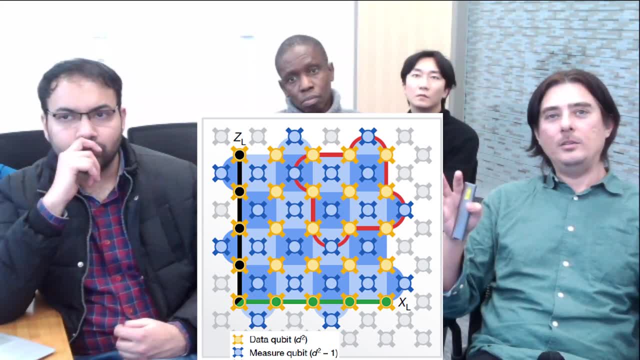 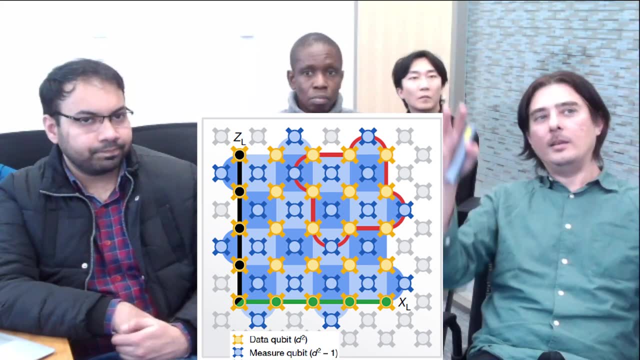 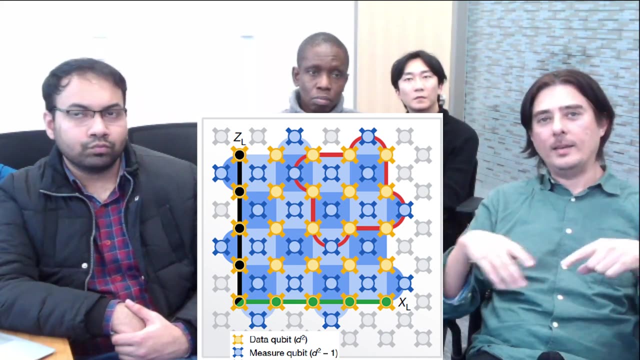 The actual surface code that they use. they use kind of two different varieties, So the five by five, the yellow ones. that's basically one configuration that they use, And so there are 25 qubits that are actually encoding the actual state. 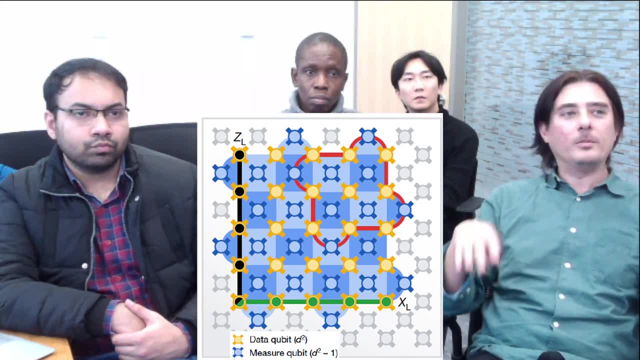 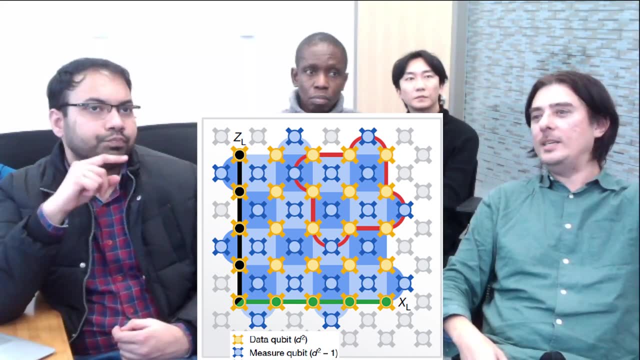 And then there's 24, the blue qubits. if you count them up, there'll be 24.. Those are used for the measurements. And then so Manish, the one, the thing that you mentioned- for the two Zs. 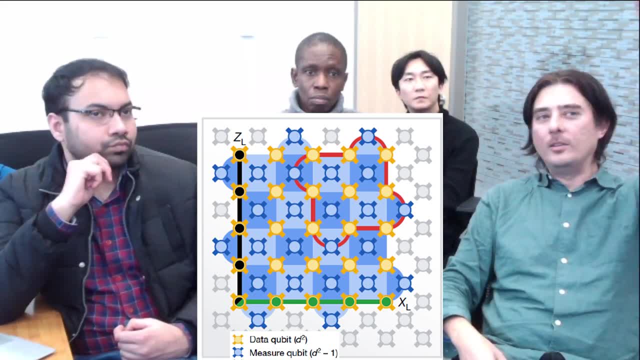 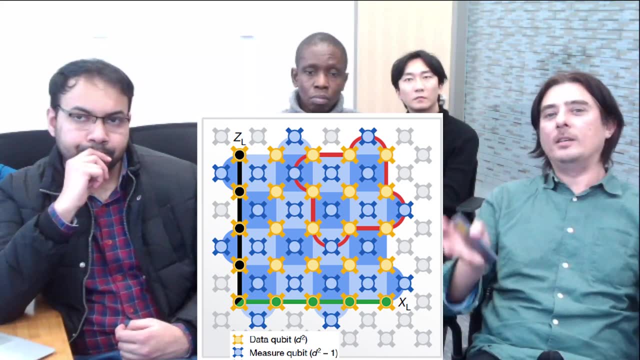 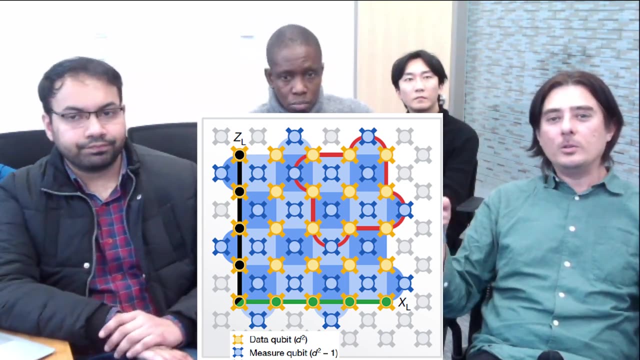 so those things that are sticking out on the sides there, those are actually measurements to do with, like, say, two Zs or two Xs, And all this encodes just like one logical qubit And the way that you can actually read out the logical information. 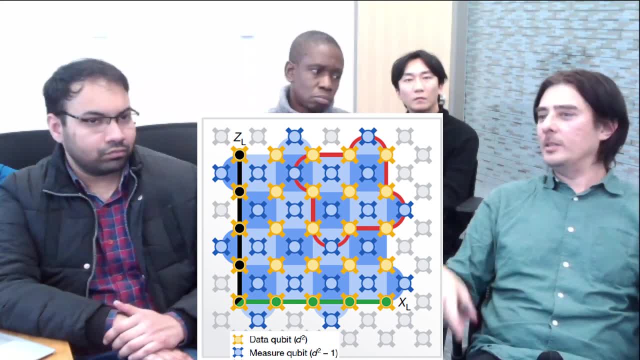 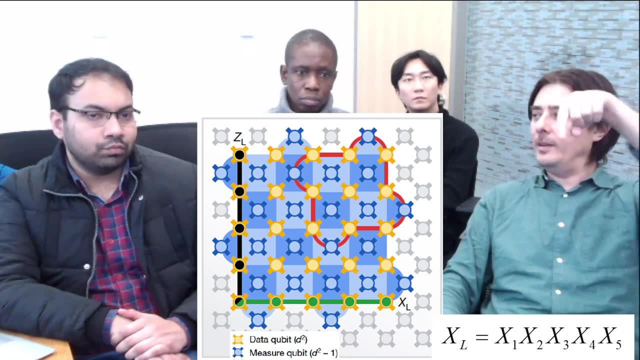 is that actually you do either a X measurement or a Z measurement, And so the green line that you see on the bottom there, if you measure in the X basis, all those five there, multiply them all together, then that will be actually your X readout. 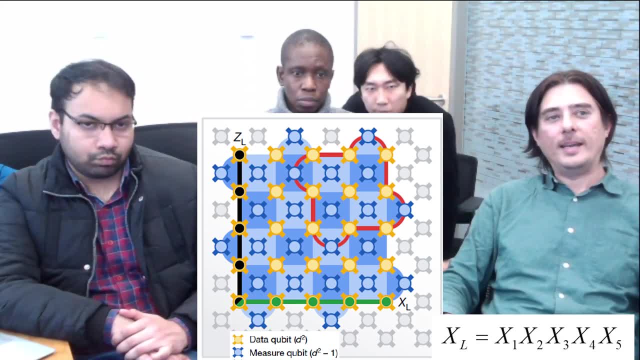 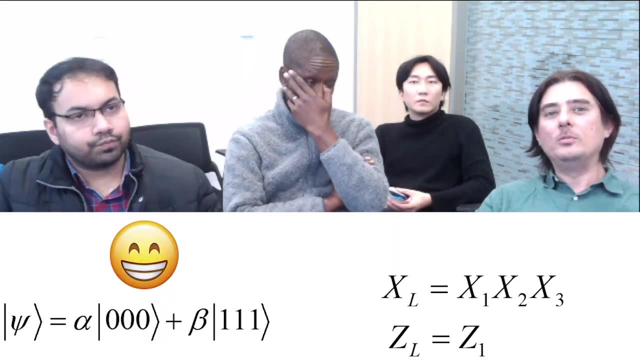 So your logical measurement is actually just that, And this is something that we also saw in the ordinary bit flip code, For example. if you wanted to know what the logical X of this encoded state is, what you'd do is you'd actually calculate. 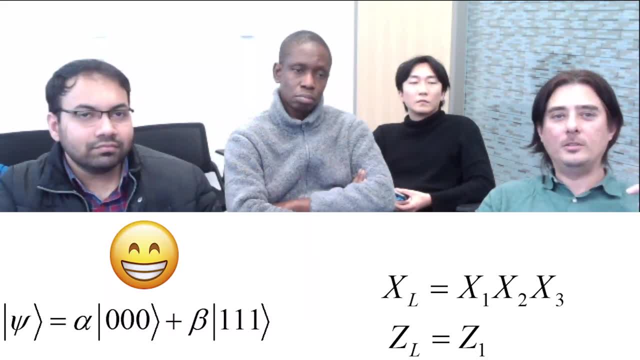 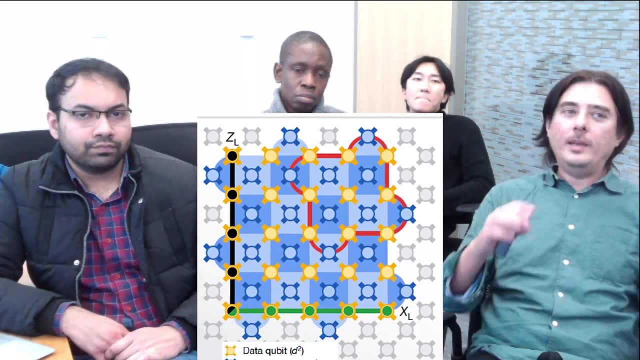 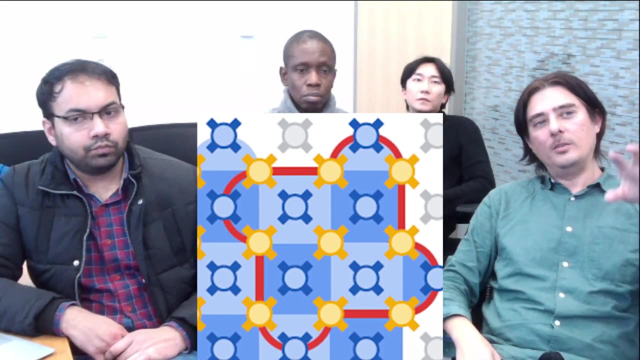 the expectation value of XXX, And then that actually gives you the X readout. In this case, the Z logical is just any one of those Zs And they compare it to like a smaller surface code, And so they have a smaller patch of this surface code. 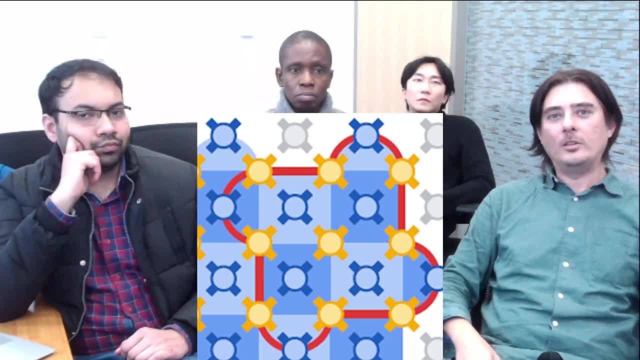 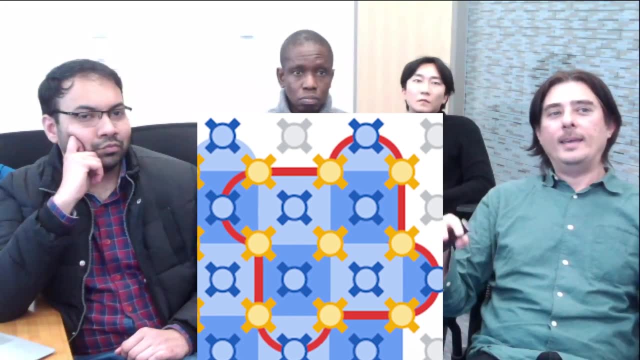 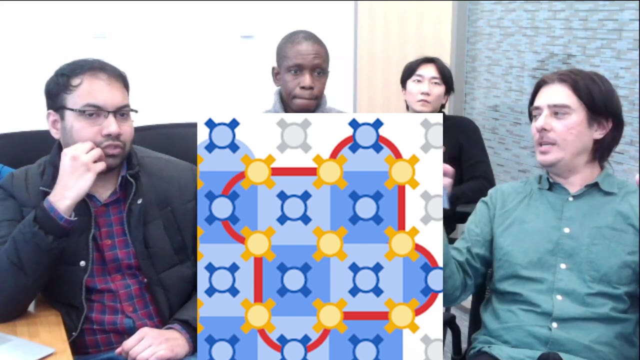 That actually makes up like a three by three surface code. So there's nine surface code qubits. You need eight ancilla qubits in order to do the measurement, And then that again is one logical qubit. The logical X operation would be a string of three Xs. in this case. 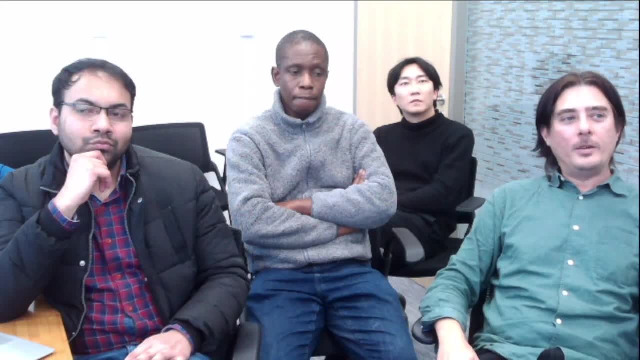 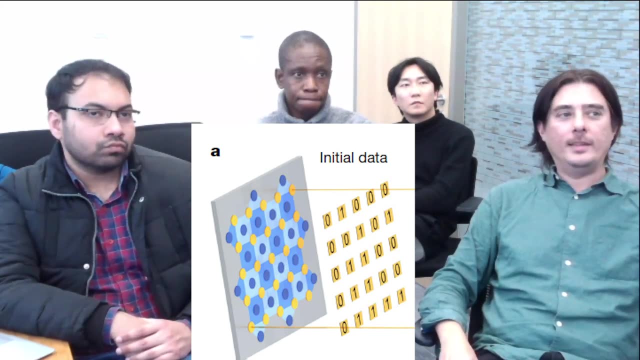 That's basically the setup, And so what do they actually do in the experiment? Well, what they do is they first start off by preparing the surface code, And they do this basically by first initializing a bunch of qubits which are in the Z basis. 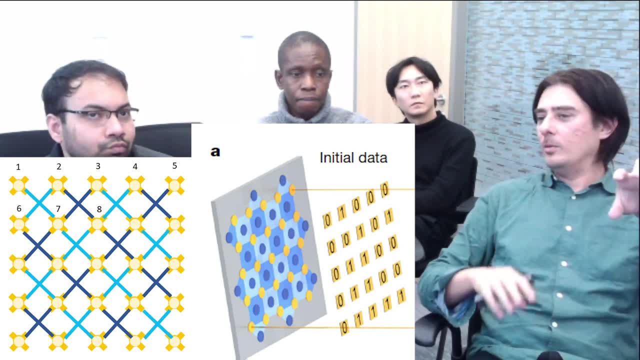 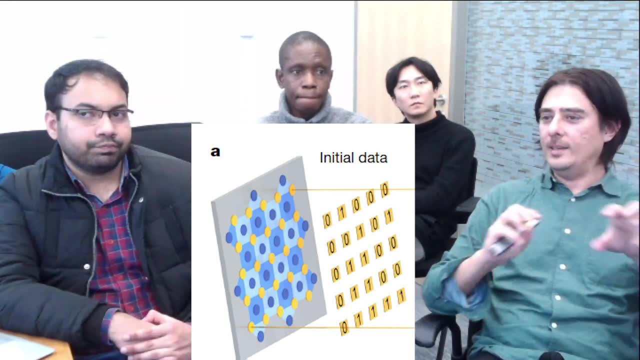 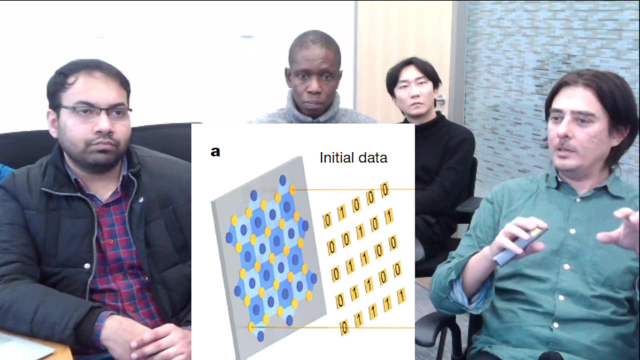 And then they keep on applying either the four Xs or the four Zs, And they do that by doing that circuit which I showed. So basically, that's continually projecting it into this same surface code state. So ideally, if you do that in a world with no errors, 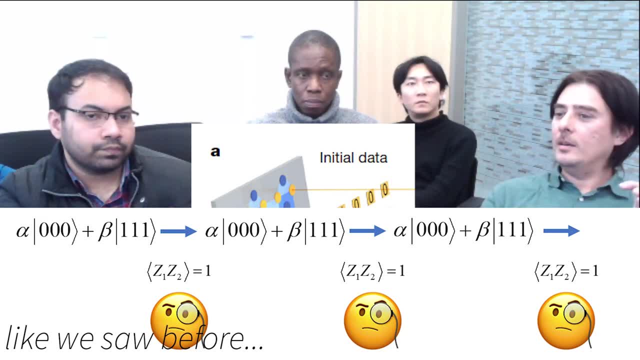 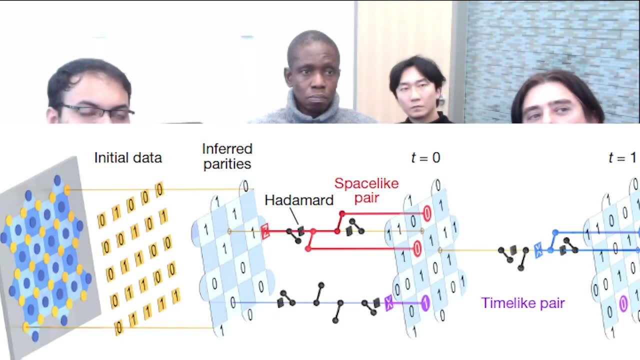 you'll just keep on getting some particular readouts For each of those four plaquettes. each one of those gives one measurement, And so the blue and light blue checkerboard that is, for example, is like the ideal readout of the surface code. 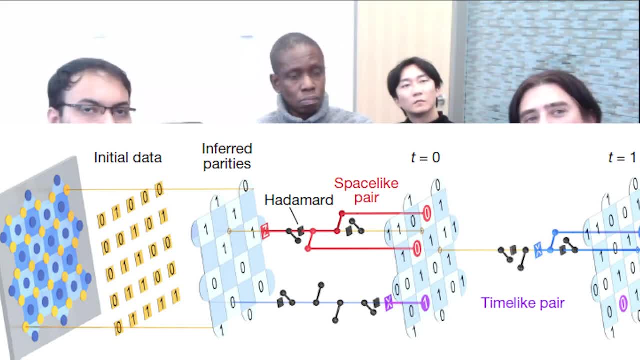 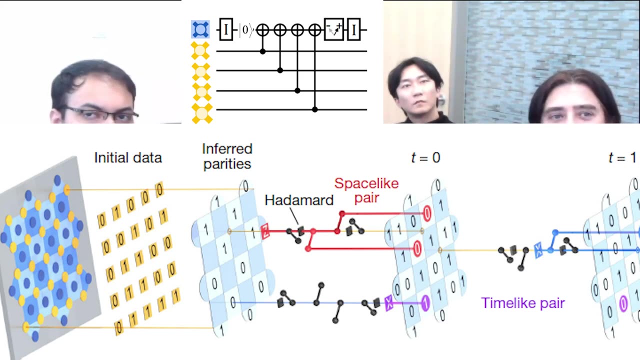 Now from there, say an error happens on the first one that they show here in the red is actually an error happening on one of the yellow qubits. Then they're continually doing that circuit with the four CNOT gates. Then what happens? because you have these CNOT gates, 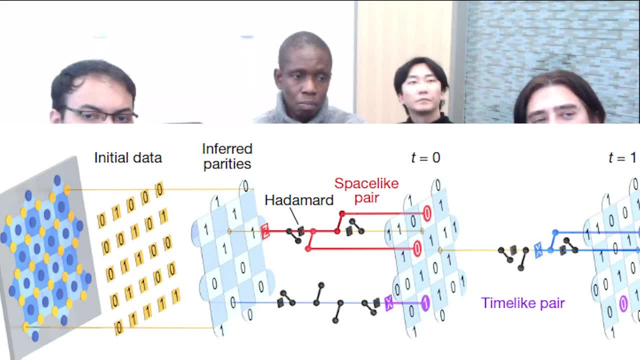 the error due to that initial Z error actually kind of spreads out And so that error is seen on potentially two syndromes. So the two red outputs there that you see at t equals zero here are like two errors that will happen because you can trace it back to a Z error. 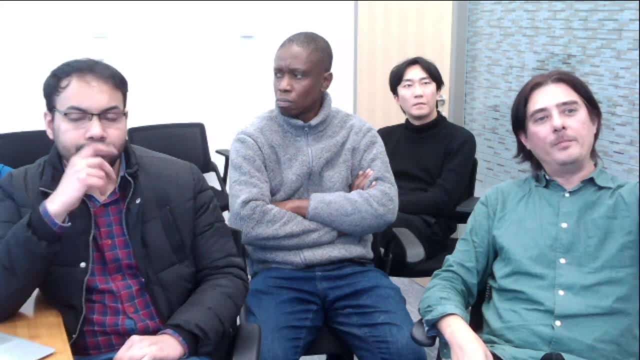 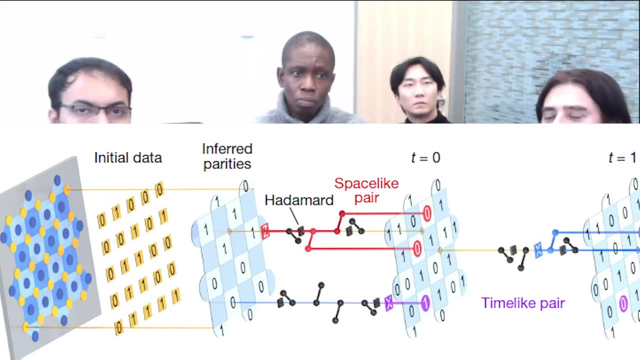 happening on one of the yellow qubits, The purple one. here is a case, for example, where an error happens on one of the blue qubits. That's one of the measurement qubits And in this case you get a circle time like pair. 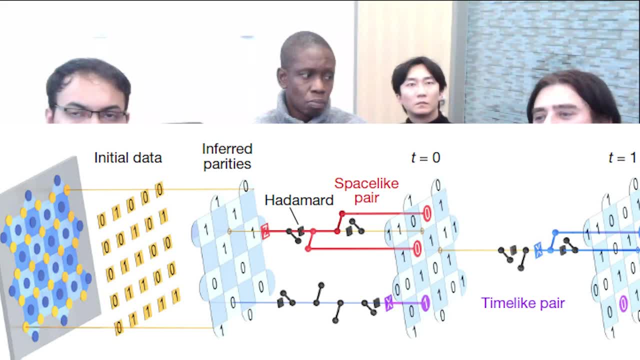 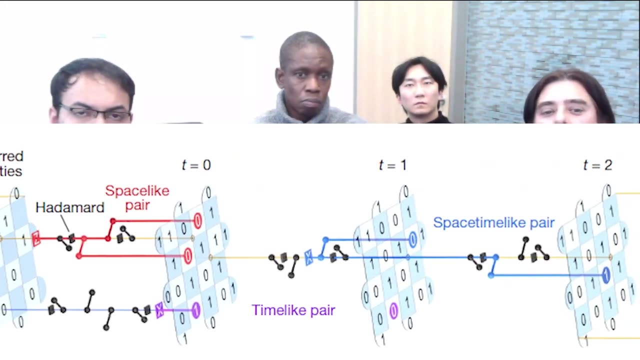 which basically means that there'll be some change in the syndrome from one time step to the next time step. So you can see the purple one is changing from one to zero, And so that's the kind of signature of that type of error. The blue one is if an X error happens somewhere between. 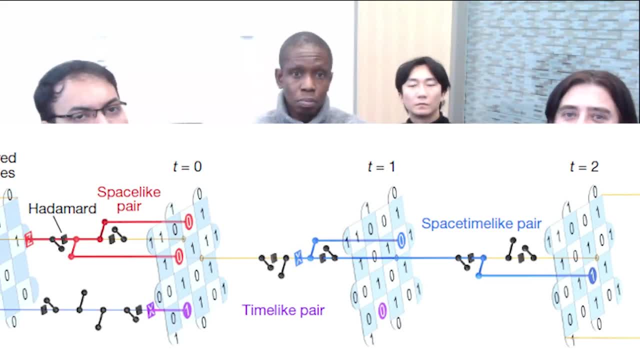 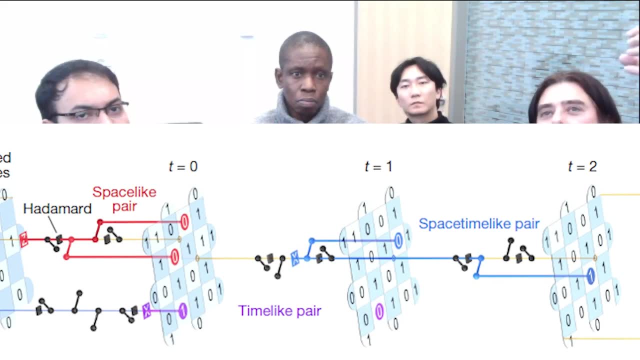 in the middle of that quantum circuit when you're doing that measurement And then in that case you get like an error that changes these syndromes. It's separated in space in terms of the pattern, but also between two steps in time. 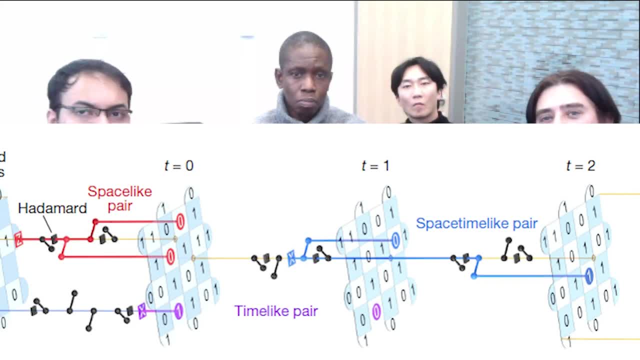 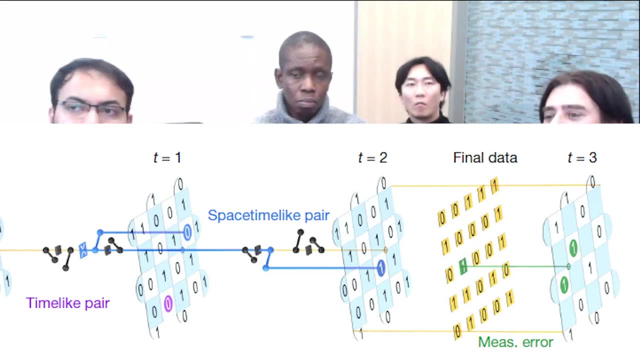 So different types of errors have, like, different signatures, And then finally they go and measure the whole bunch of qubits either in the Z or the X basis And then from that they can kind of infer something about the logical state of the whole thing. 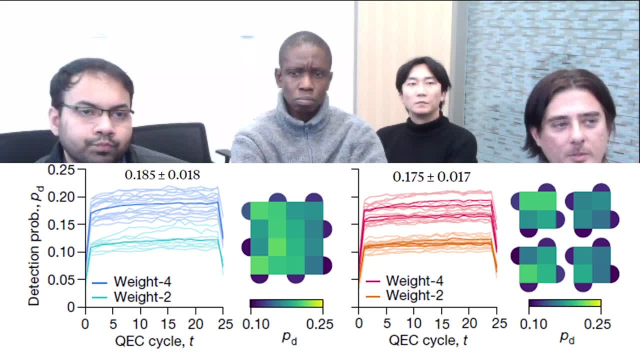 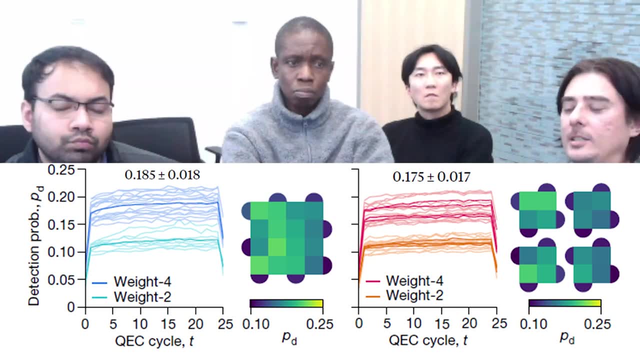 Okay, so what do they actually see in the actual experiment? So, firstly, these graphs are basically just detecting. you know what probability are they actually detecting an error, right? So basically, anytime you know you're doing all these measurements constantly. 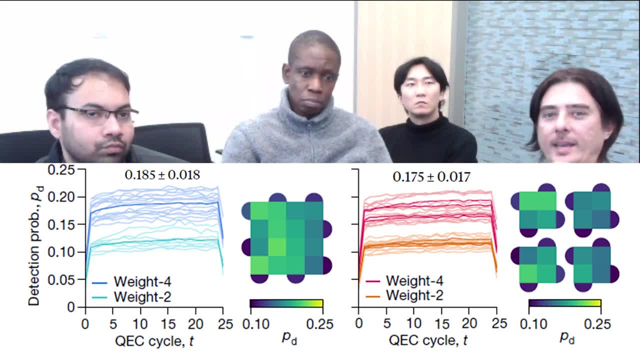 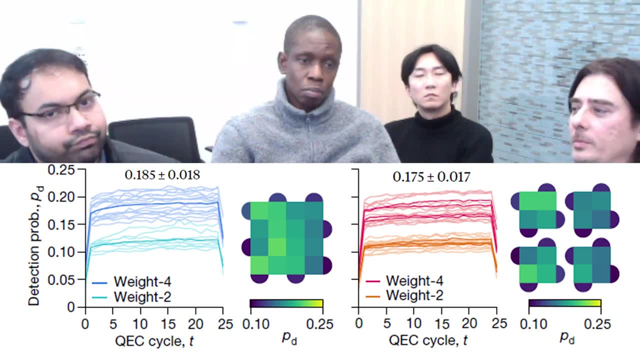 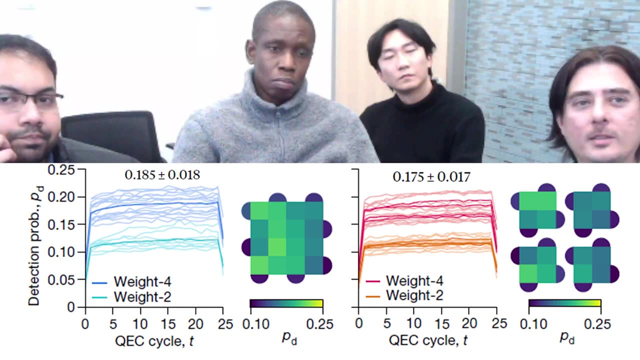 measure, measure, measure, measure. Ideally it does not change between different cycles, right, But then occasionally it will, And then. so, basically, what is the probability of any one of those syndromes changing between, like one time step to the next time step, right? 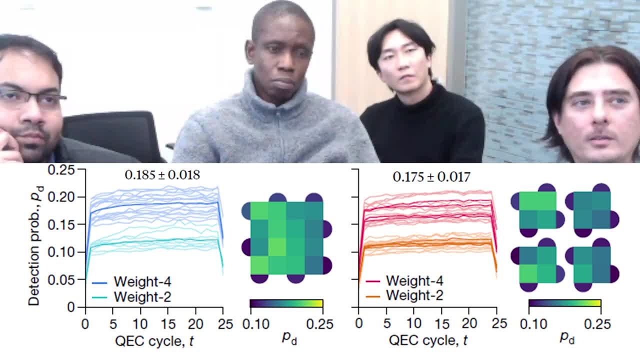 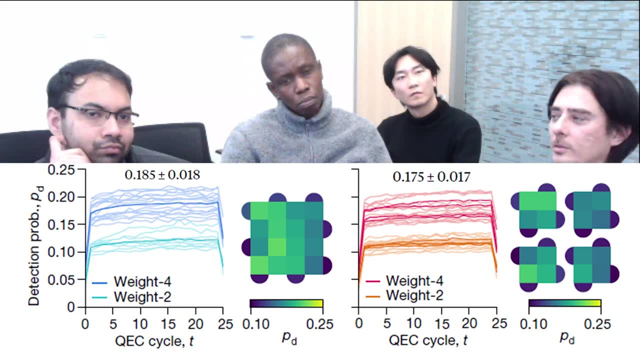 And then the probability they get is something like you know, 0.18.. So basically, roughly one in five or five or six cycles. you know you'll see some some error happening somewhere, right, Okay, And then 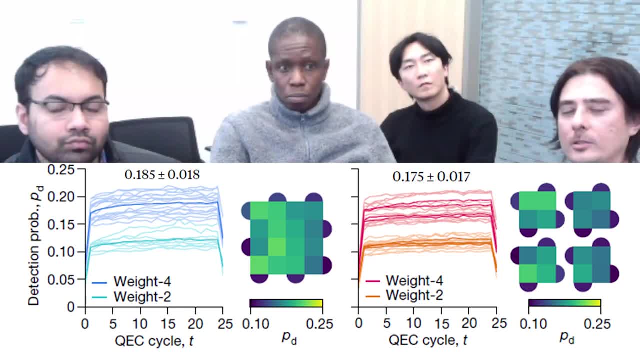 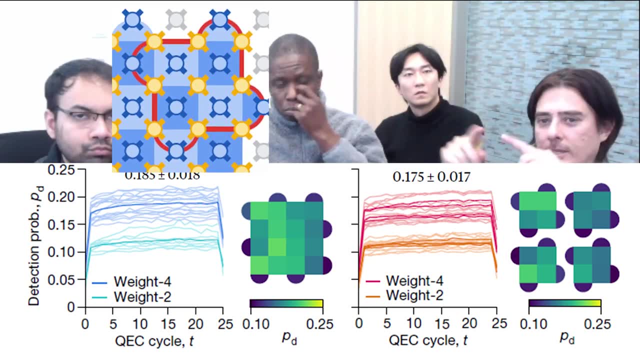 so the one on the left here you're seeing this is for that full, like five by five surface code. They repeat the experiment with like four smaller patches, like three by three, And then what they find is that it's basically roughly the same. 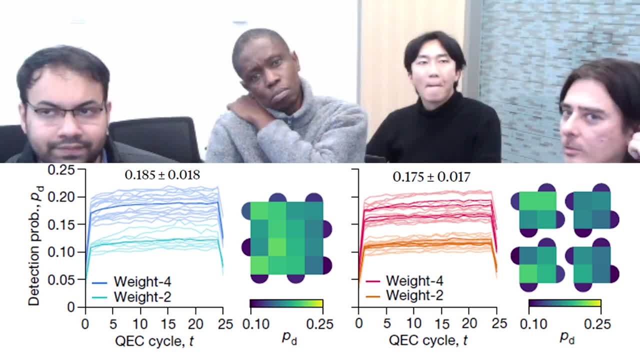 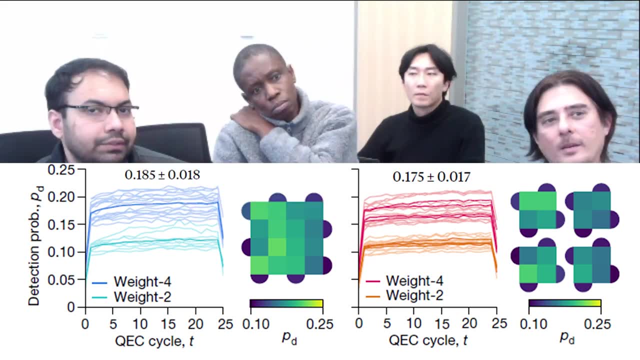 same number, I guess, because it's the same same physical system. If you're wondering what that weight four, weight two stuff is, the weight two is the thing on the edges, the thing that you were talking about. So those always have a lower probability. 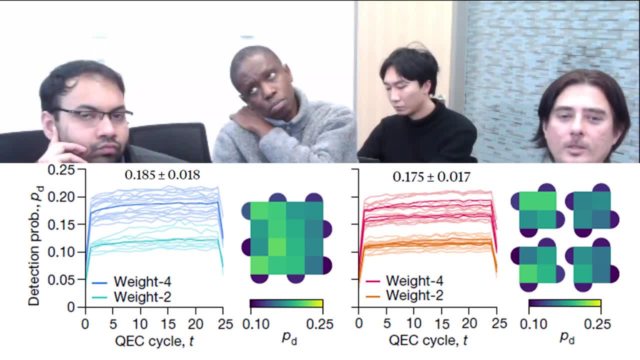 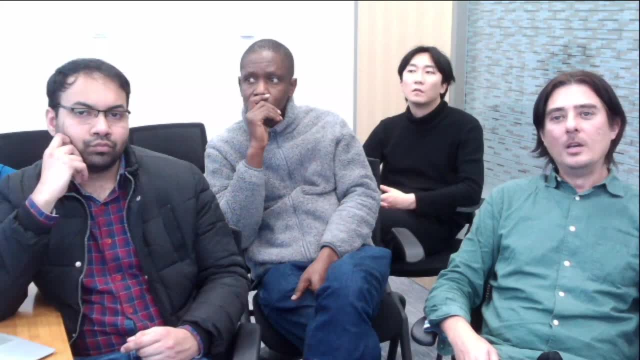 because they only involve like two, two qubits. Okay, So now coming to the main results of the paper that they really want to show. eventually, what we want to do in this whole- error correcting, you know, situation or round- is that 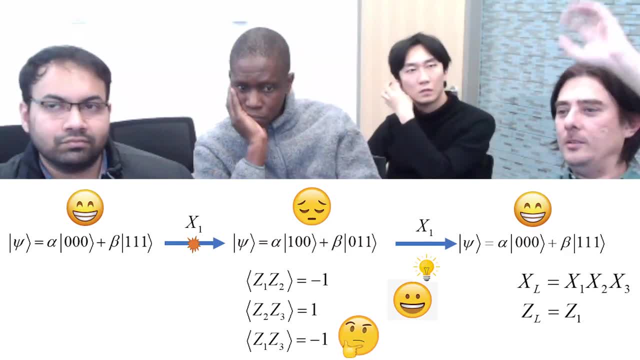 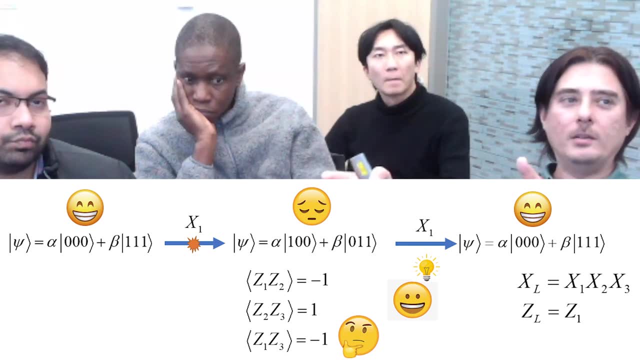 you know an error happens, you detect it and then you correct it And then you have some final state which is the final logical state. And ideally the final logical state is the same as the initial logical state, right? So? 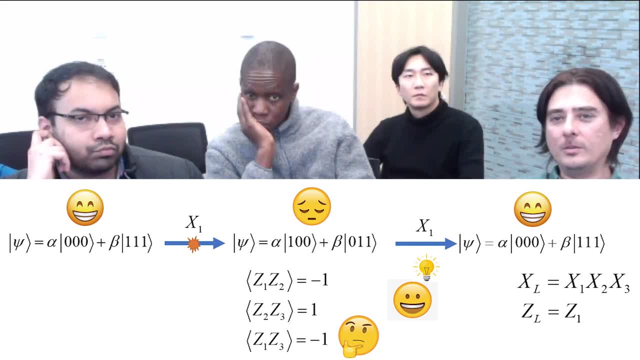 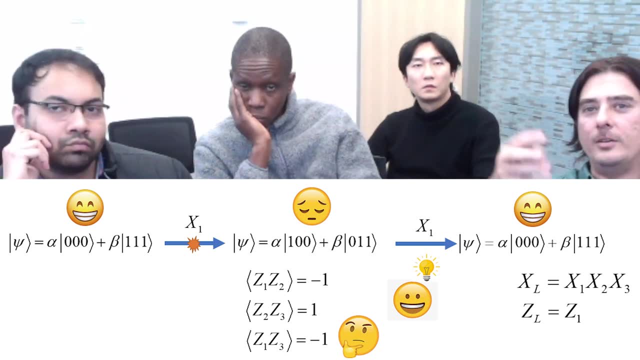 you know you want to compare the sort of the input to the output and basically make sure that it's the same. Okay, So firstly, actually they don't actually literally do this X correction. They don't actually apply like another gate in order to make the final X correction. 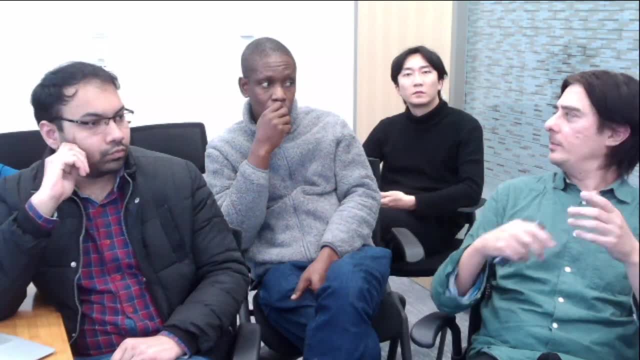 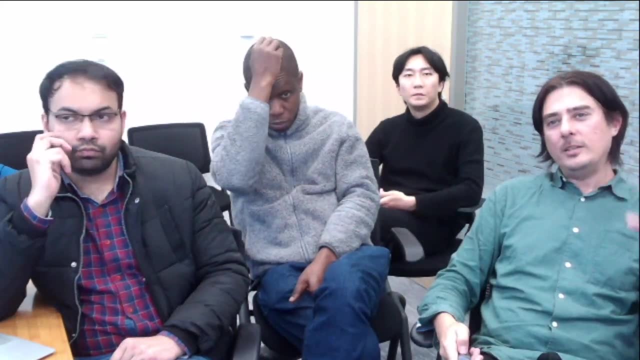 And I think that's because, basically, you can always account for this just by some post processing, So I don't think they literally need to actually account for it. But actually, what's more, it's not quite as simple as what you think. 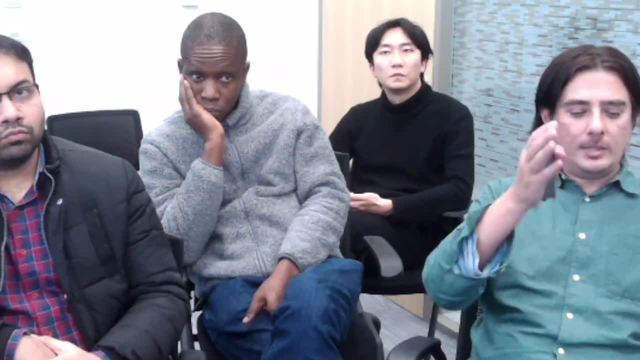 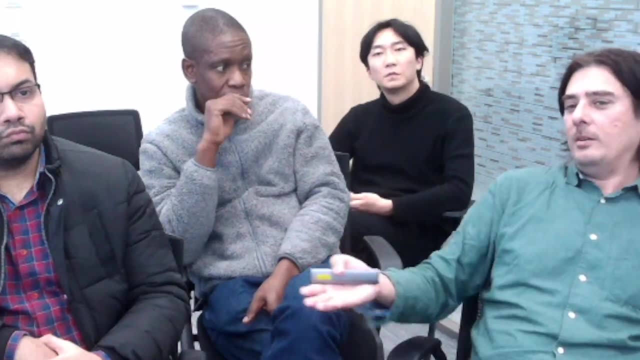 because what you would think is that you know, okay. so you start with the state and then you end, you measure the final state and then you compare the two and you know. you just see how different they are, right. So 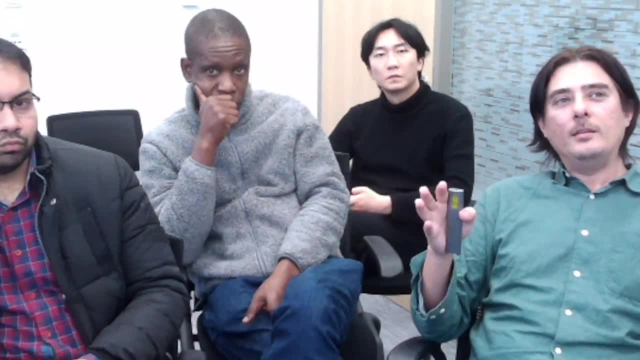 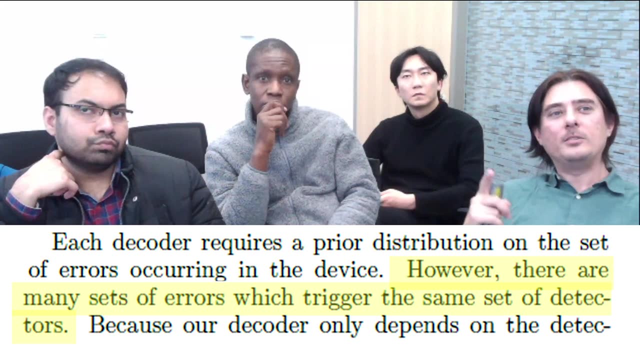 you know, just do some kind of fidelity, But it's actually not what they do, And if you read the paper carefully- and this is from the supplementary information- they say something like this: that, however, there are many sets of errors. 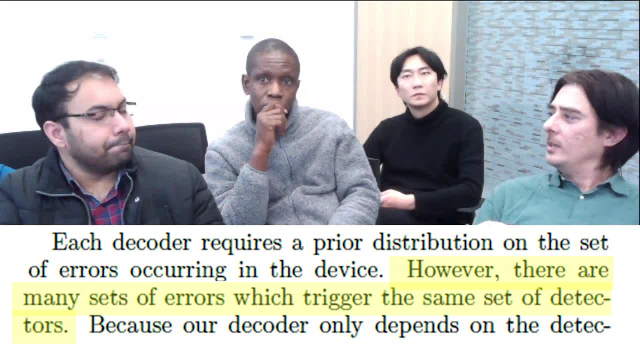 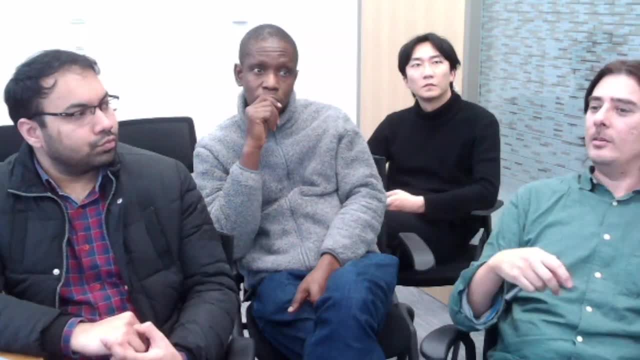 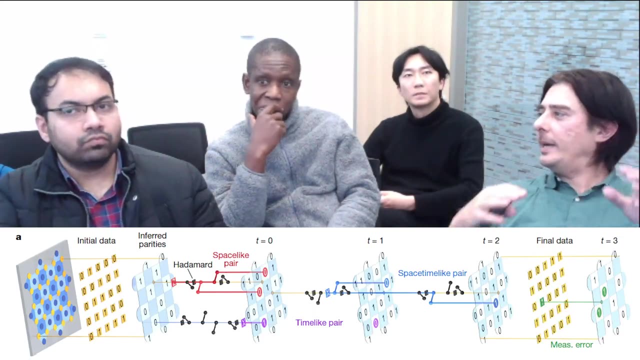 which trigger the same set of detectors. So that basically means that when they detect errors, they can't exactly pin down exactly what error it was. So remember that whole story with the different errors making different patterns. Apparently, this is still not sufficient. 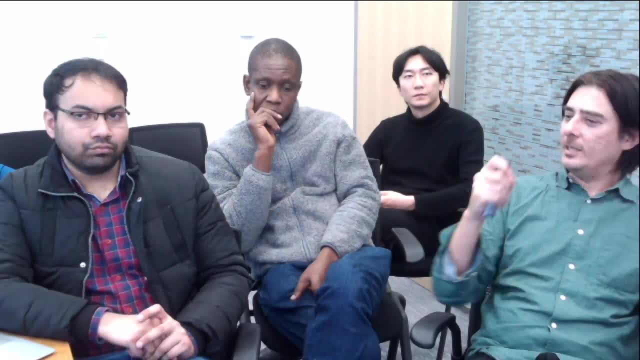 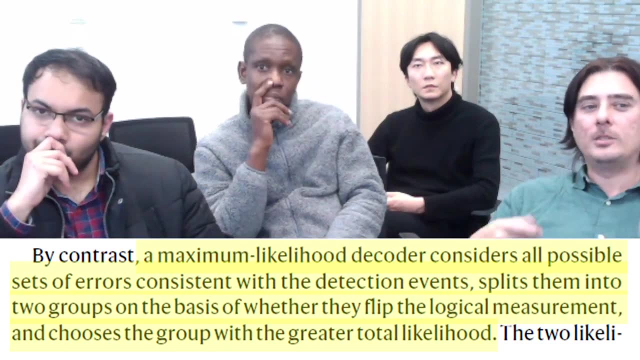 to actually figure out exactly what happened, because if they knew exactly what happened then they could go and correct it. But apparently there's insufficient information. So what they actually do is some kind of maximum likelihood estimate of given a particular error detection result. 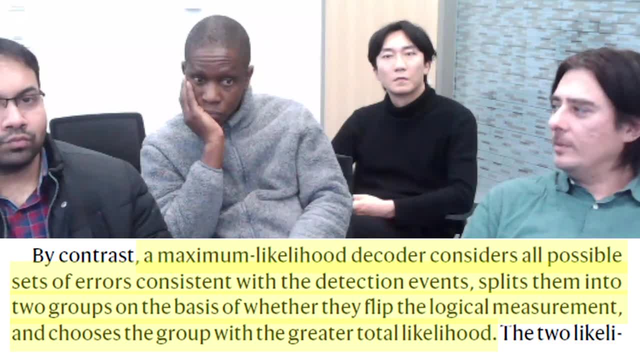 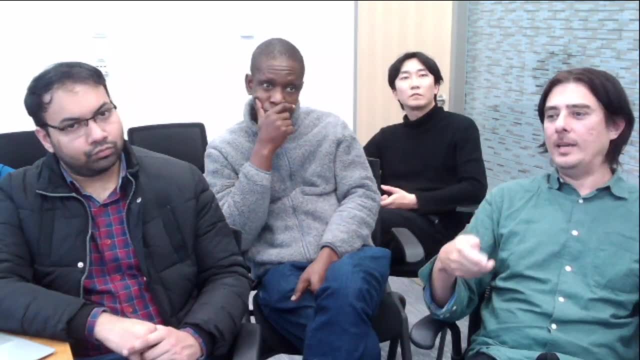 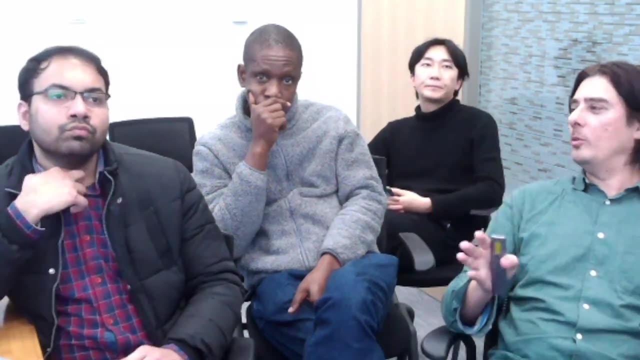 what is the most likely thing that happened, and then make their correction based on that. And then what they do is they from there basically estimate what is the actual probability of a logical error actually happening. So what they do is actually a little bit more complicated. 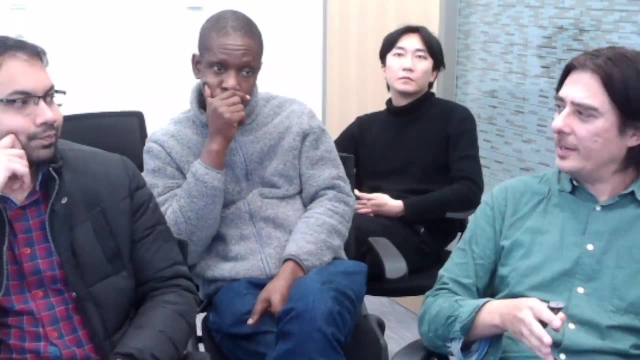 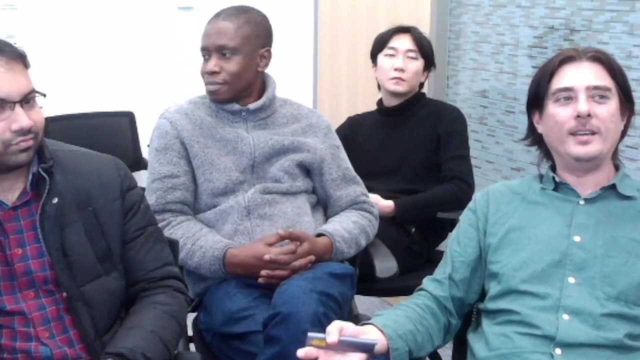 It's not quite as straightforward as you would like, because you know you would like straightforward comparison of input, output. compare it, Okay. so how good is this thing actually working? Anyway, so that's what they do. So in the vertical axis: 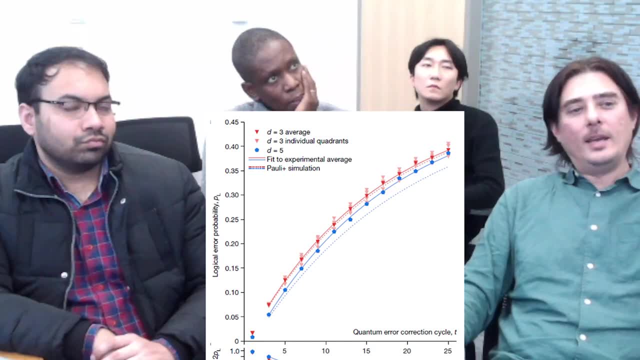 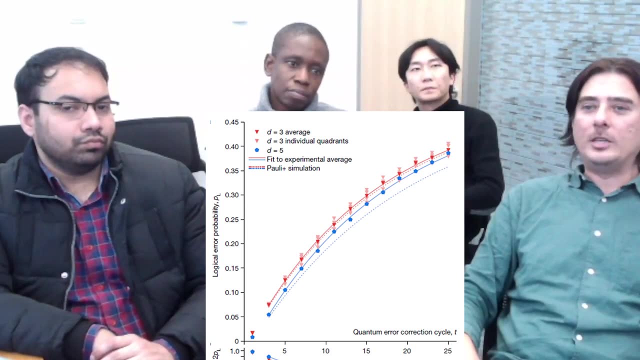 what they show here is the logical error- probabilities- and horizontally, the horizontal axis is the number of cycles. So these are all the number of times that they're doing the full set of measurements, And what they basically are seeing is that, as you do more cycles, 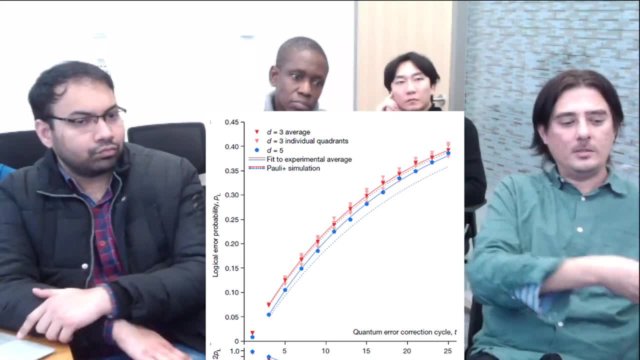 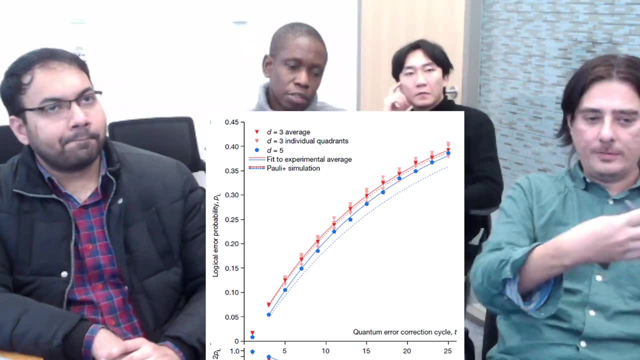 obviously this is cumulative right, So it's the same system and you keep on applying the measurements, And so if there's an error that occurred in the first step, then after more cycles there could be another one, and another one, and another one. 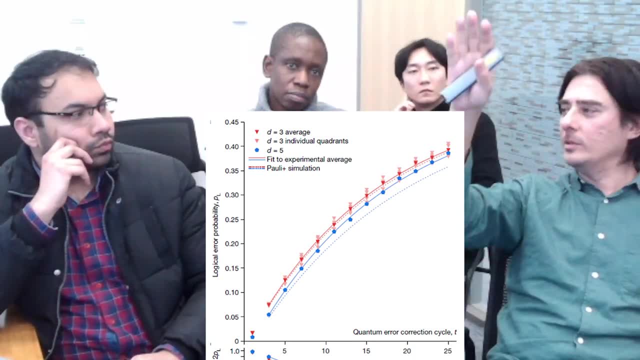 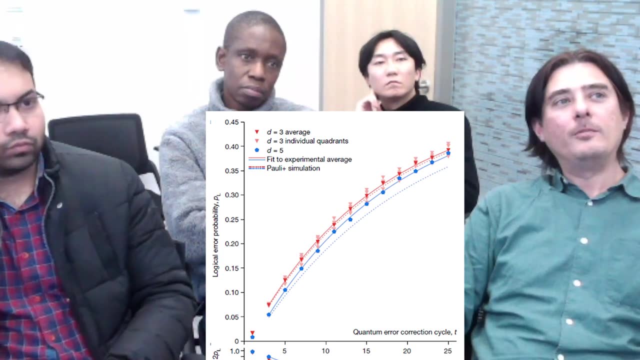 And so the probability of getting some kind of error of course increases. Okay, but the key point in this first one is that if you look at the line for the smaller codes, so the D equals three, that's the three by three surface code. 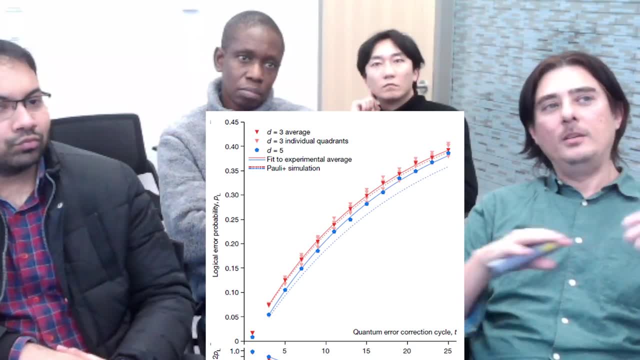 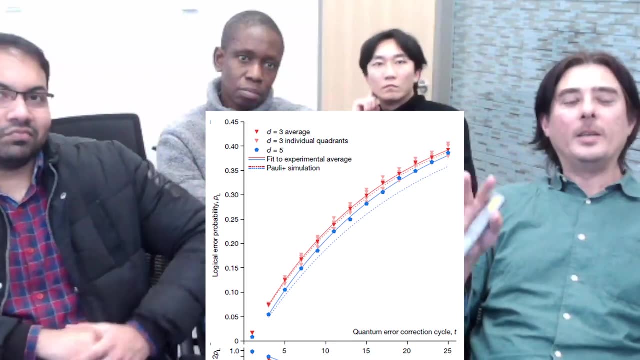 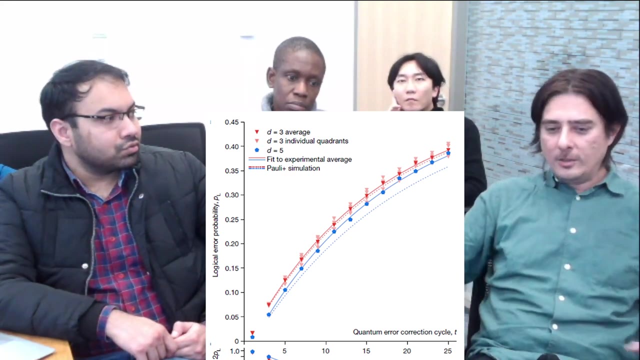 it's actually higher than the probability for the larger surface code. So this is kind of the result they were trying to show, because what should be happening is that, overall, there should be a benefit of using the larger code In the larger code. yes, of course. there's more opportunities for errors coming into it because there's more qubits, But then overall there should be a net gain And this is the whole idea of fault tolerance and stuff. So as you increase the size of the system, you should be benefiting. 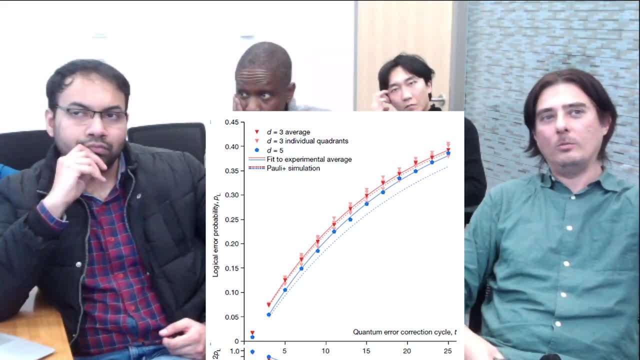 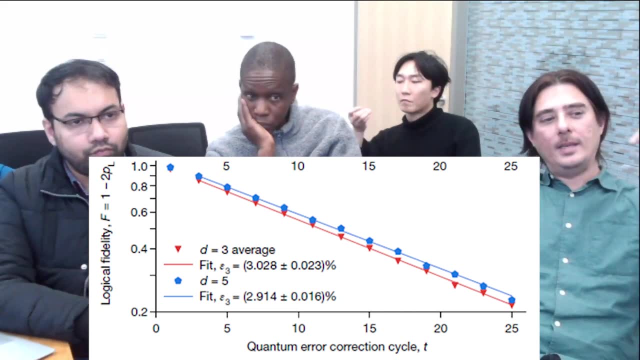 by doing so, And so this is basically one of the key results that they're showing. The bottom one is basically just kind of fitting this same thing to an exponential, but then looking at the probability of getting an error per cycle, The gradient here is: 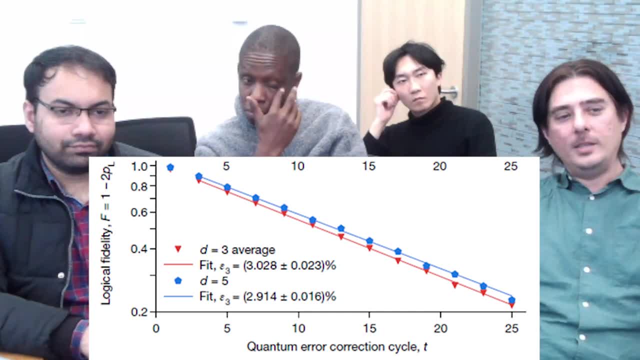 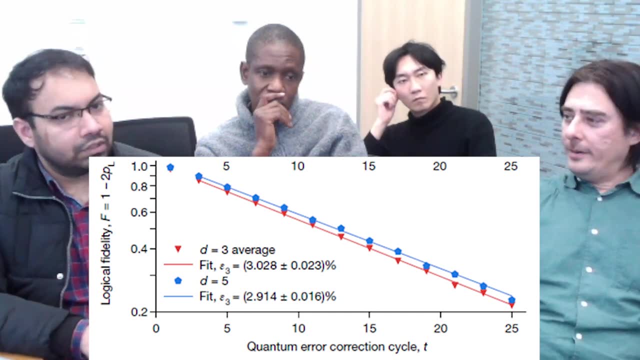 so the 3.28% that you're seeing there is saying that okay. so per cycle there's a probability of 3% of getting an error, a logical error. Compare that with the larger one, which is the D: equals five. 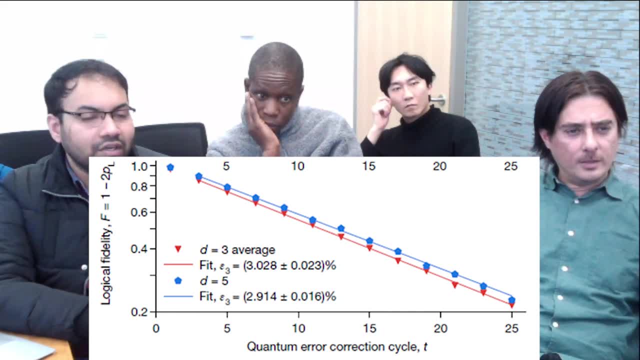 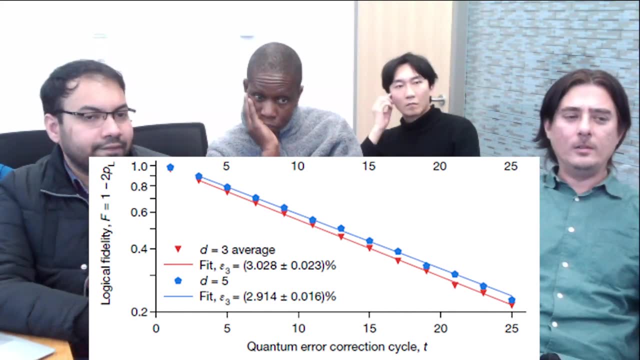 I think that should say epsilon five. right Must be right. Yeah, so I think the epsilon five must be for the larger surface code, So that has a slightly lower error probability per cycle, So each time. So this is sort of. 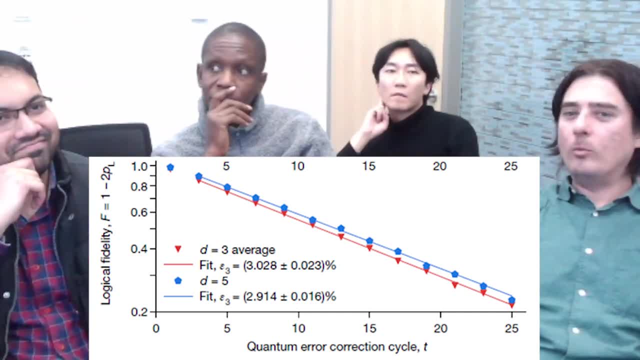 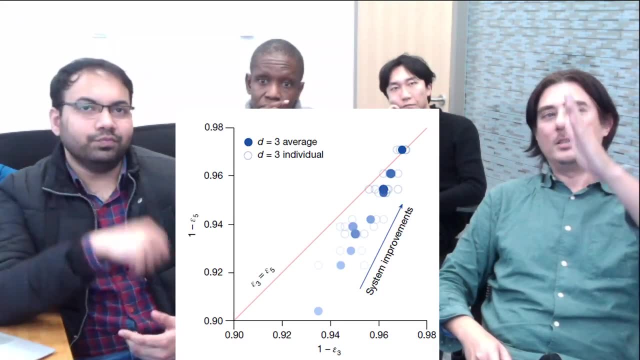 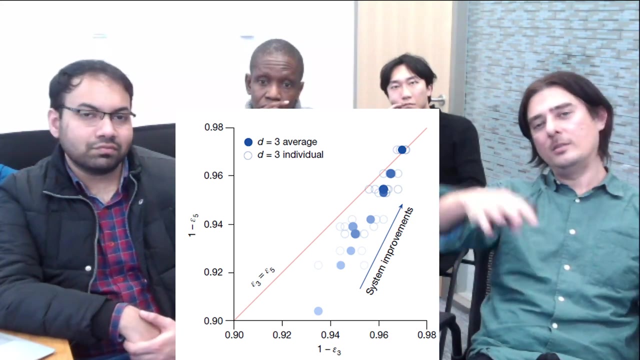 the money shot result that they want to kind of show. They also showed, like, the experimental progress, actually, in order to get to this point where the three by three surface code is not as good as the five by five In all their previous experiments. 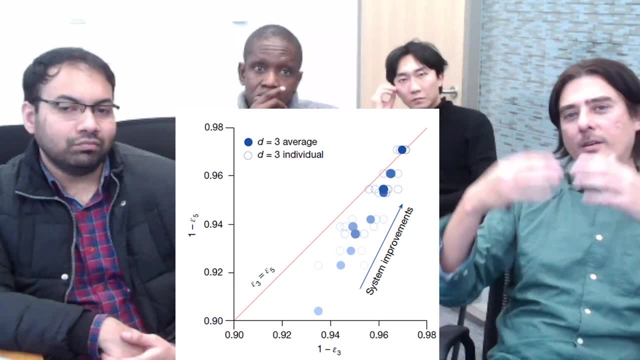 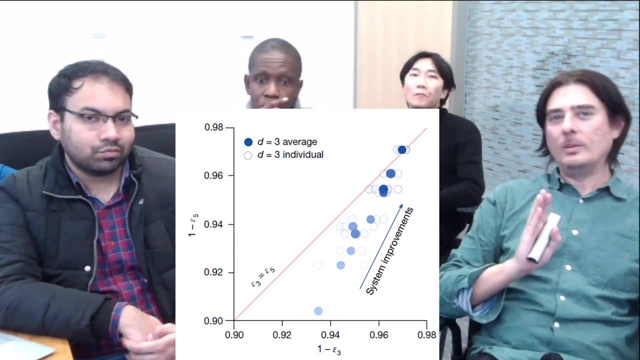 the three by three was always better than the five by five, but with various improvements, the five by five has finally overtaken the three by three, And so I guess what this is supposed to imply is that you know as they? yeah. 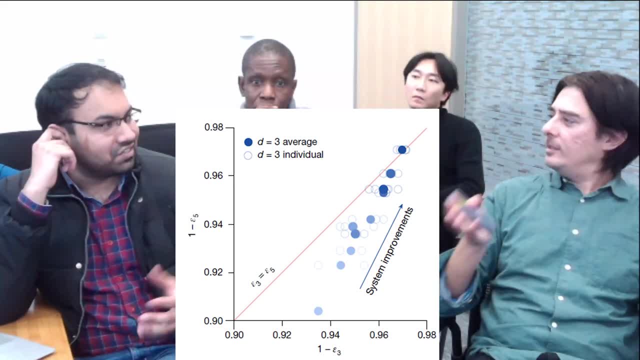 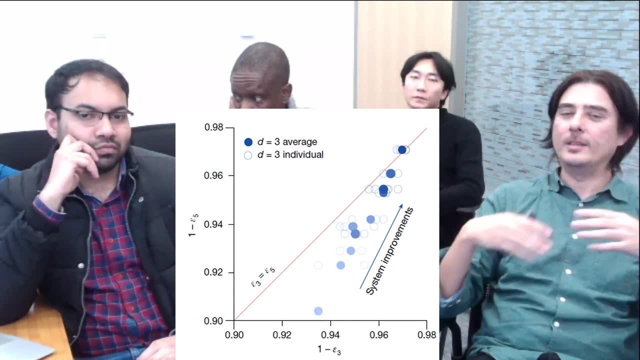 as they develop their- you know technology more. this, the five by five, will definitely become better, But this is the first time that this has overcome that comparison. Finally, this is the they also do, actually just the regular bit flip code. 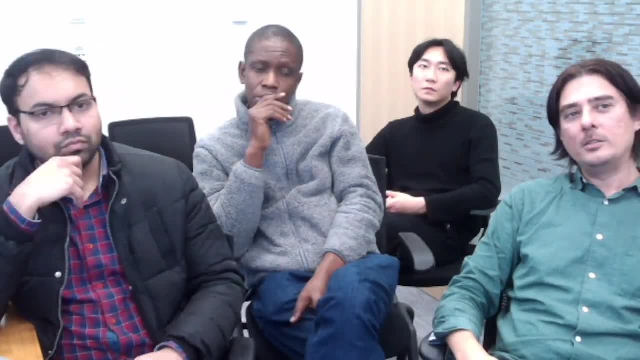 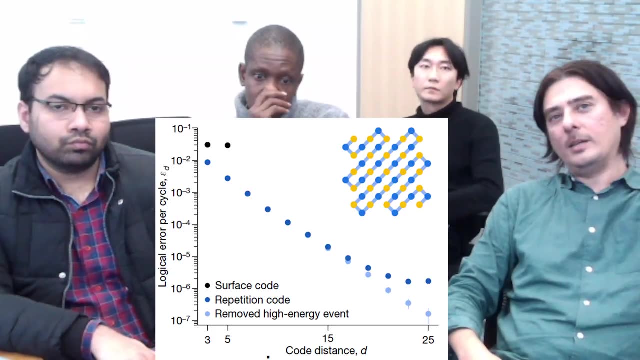 So this is the first time that this has overcome that comparison. Finally, this is the. they also do actually just the regular bit flip code, And they do this kind of snake kind of configurations using, I think, 25 qubits. It'd be like a bit flip code. 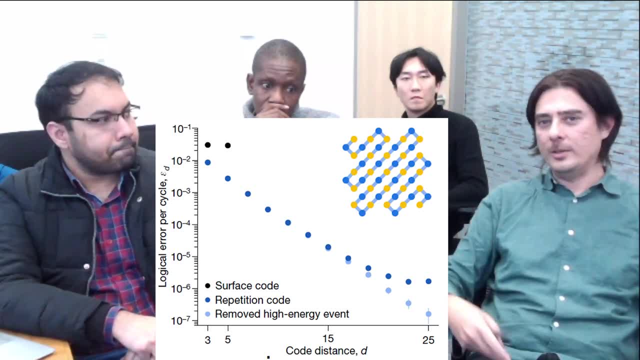 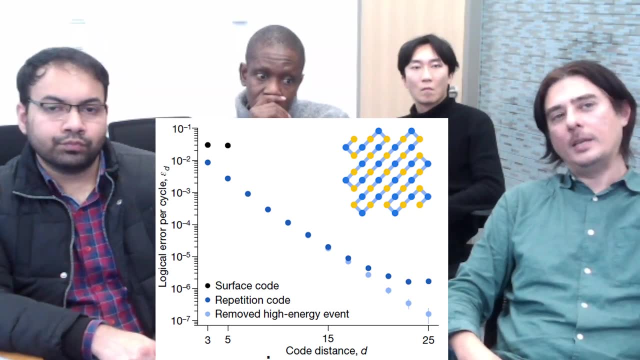 where, instead of three qubits, it's like 25 qubits, right? And what they show is that, basically, this logical error per cycle, the same quantity that we're calculating there, is actually dropping down to very, very low levels as you go to. 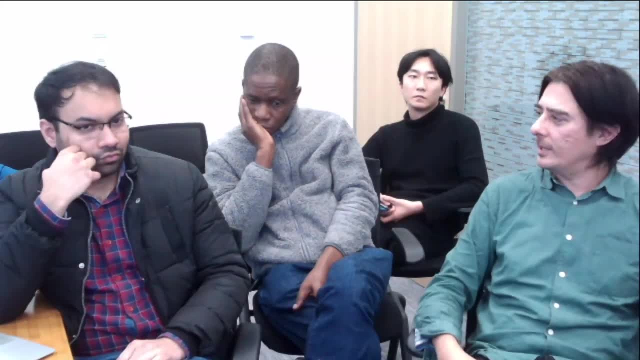 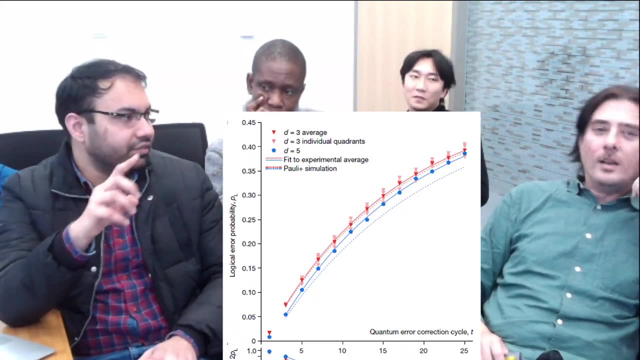 very large code sizes. They have some other results, but I think these are the main things. So what do you guys think? I mean, are you impressed? I was checking that plot where they compare D3 and D5.. So, in terms of 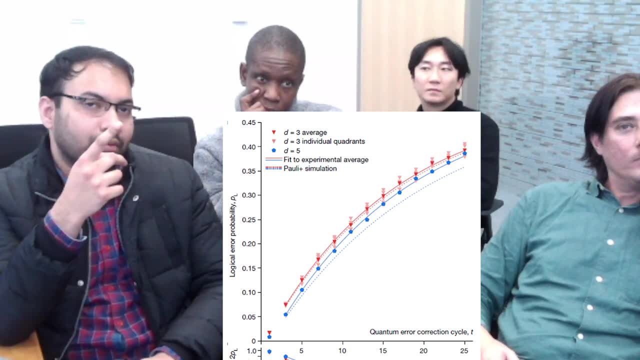 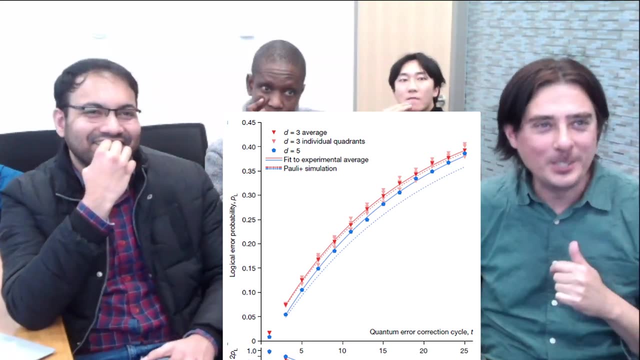 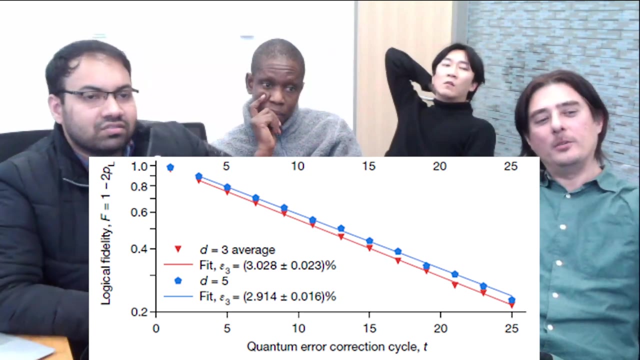 I think numerical values. how much is the improvement, Like how much percent from D3 to D5?? Well, it's pretty small. Yeah, it's pretty small, It's just a couple of percent, right, I mean in the error per cycle. 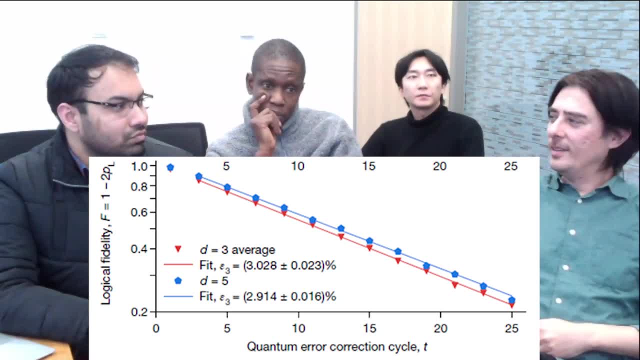 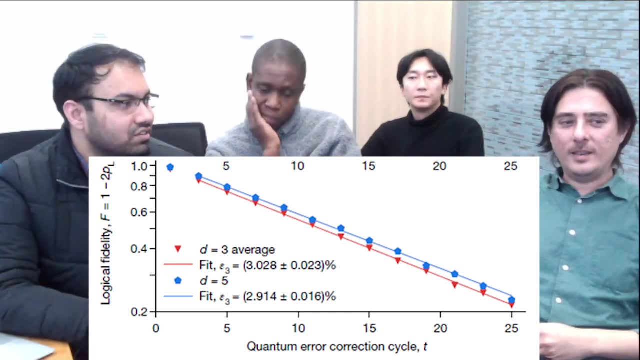 you know it's 0.1%, So it's pretty marginal, But I guess it's the first time that it's Larger surface coding. Yeah, The large surface code beats the small surface code Because if we do the scaling for larger qubit. 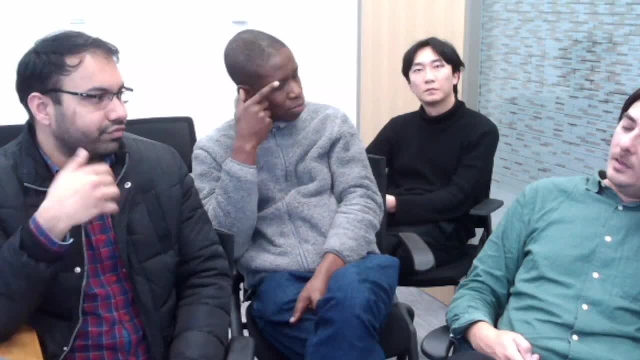 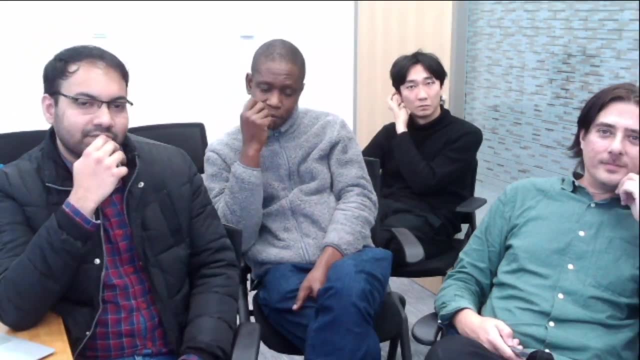 and they say 7 by 7 may further improve over 5 by 5.. You would hope so, Yeah, You would hope so, right, Yeah? So, overall, I think my question would be: what is the benefit of this error correction? 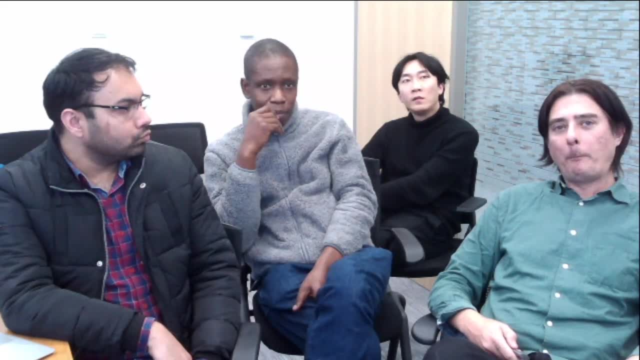 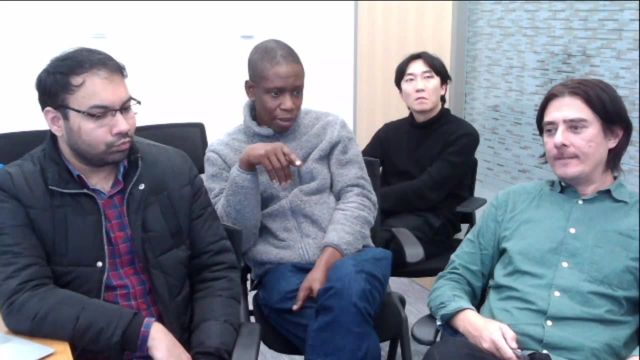 if? well, let me step back. Is there any hope of actually knowing the source of the error and correcting it as the system scales like that? Is there any hope of doing that? Well, yeah, I don't know. I was a bit surprised. 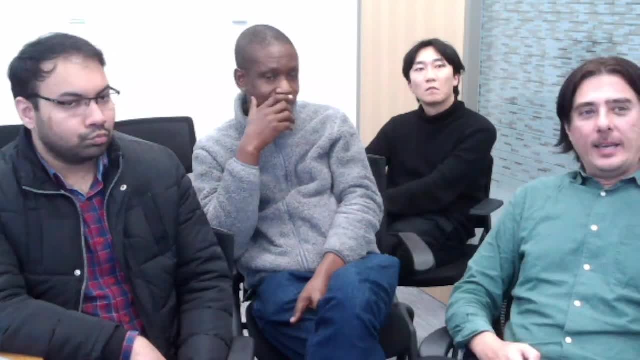 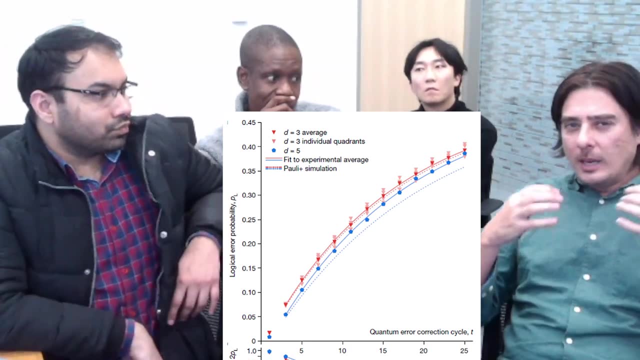 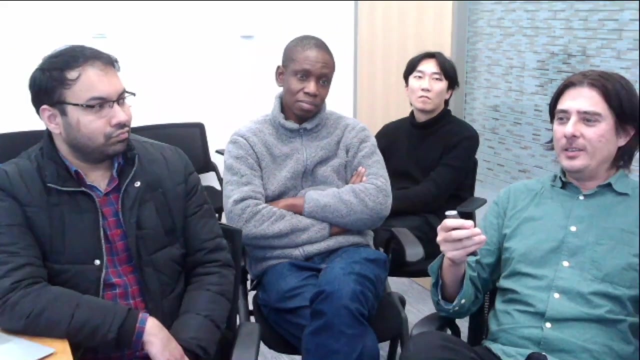 I guess that you know in this probability estimate that you know they basically still can't really pin down actually what the error is right. So the whole point of I thought, error, error, error, error correction is that 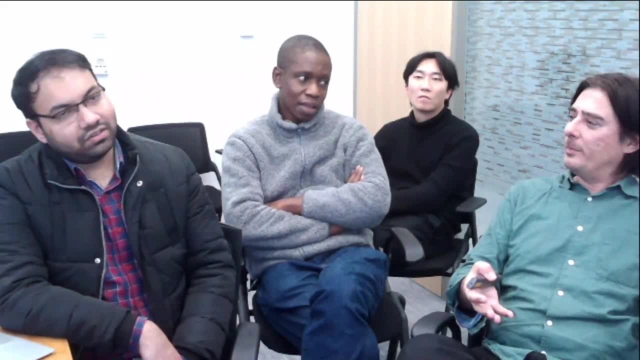 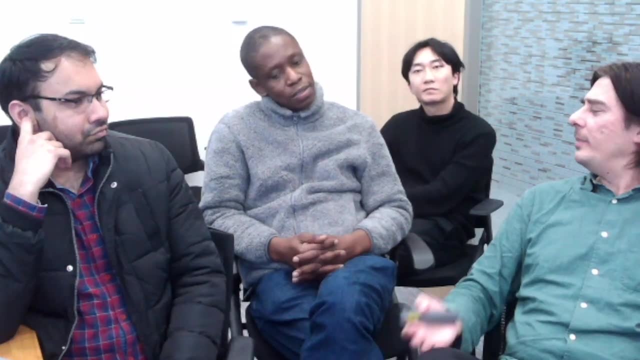 you can pin down where the error has and then you can go and correct it right. But if you can't, then I guess you need something more sophisticated, I mean, you know, maybe tailored to the system that you're doing, because 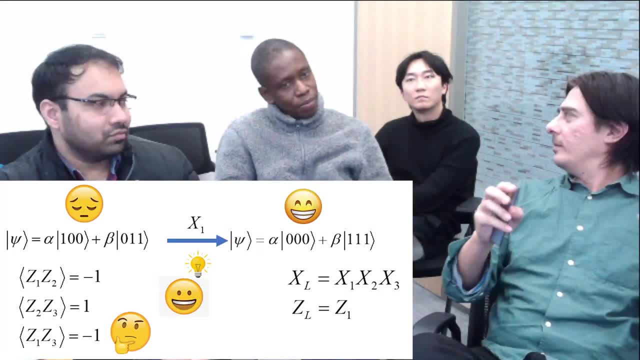 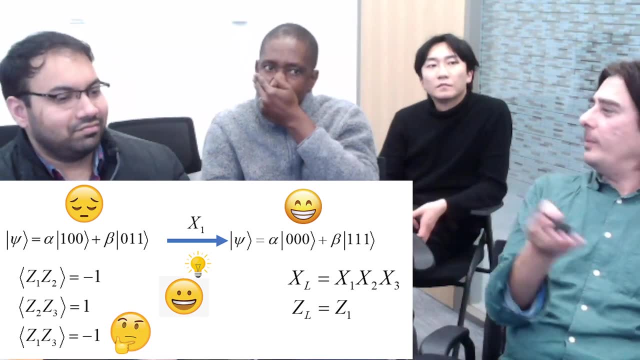 I guess the thing with this is that in my simplified example with the BitFlip code, right, you're just looking at those qubits involving the yellow qubits in this example, right, How do you actually go and measure it? But I guess what this is saying. 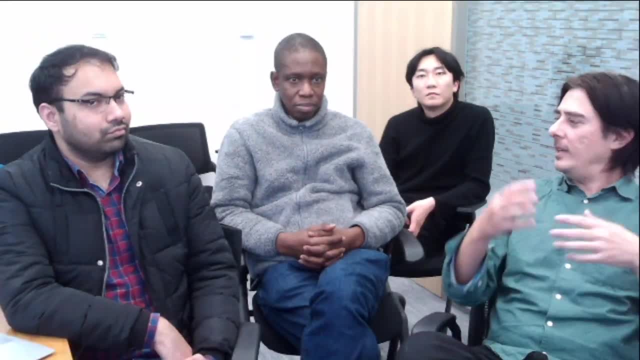 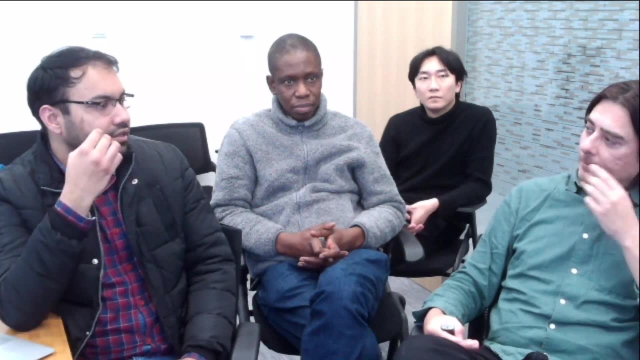 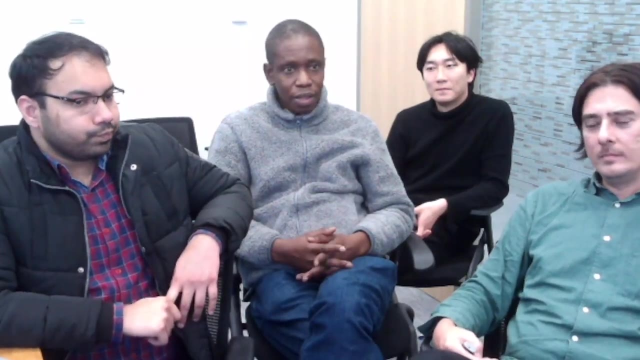 is that? yeah, the measurements themselves can contain errors and so the errors can come from many different sources. in reality, right, They use gates for the measurement that can introduce errors. Yes, Yeah, it basically comes to that. yes, Is it that? 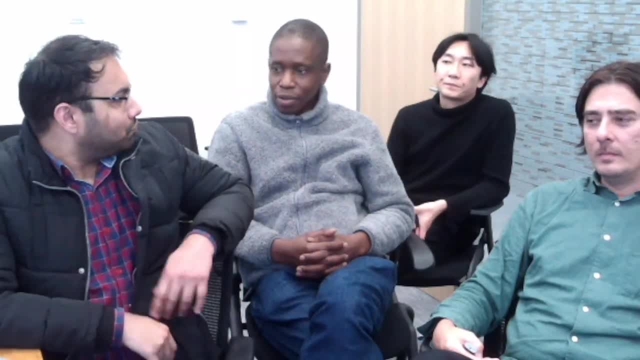 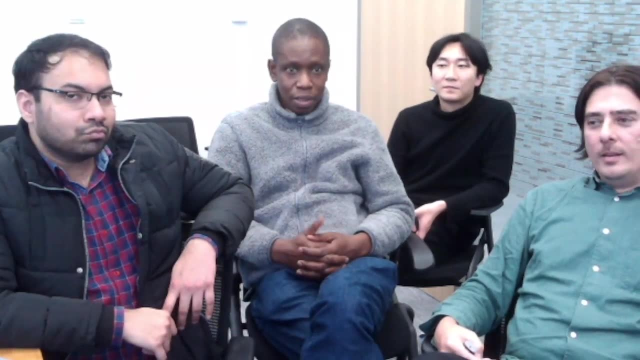 we should start thinking of better error correcting. You know what is the best strategy to do with the error in this case. I think that's what I'm trying to get at, because, because you know, naturally I would think that if you told me. 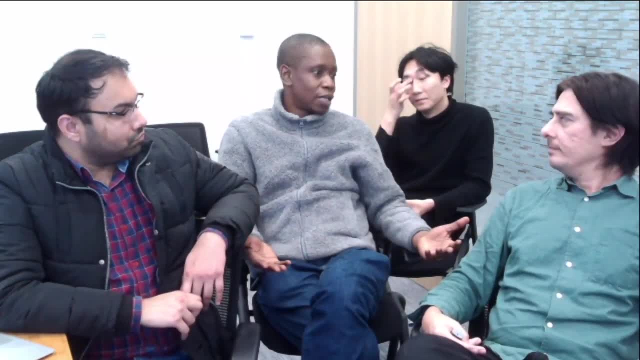 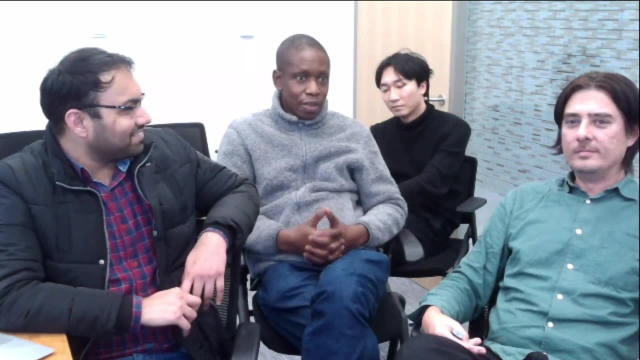 there is no error or that the error is minimal. I would just simply look at the fidelity, right, But they're doing some, you know likelihood, and blah, blah, blah. and so what is the best strategy now to track error in the quantum systems? 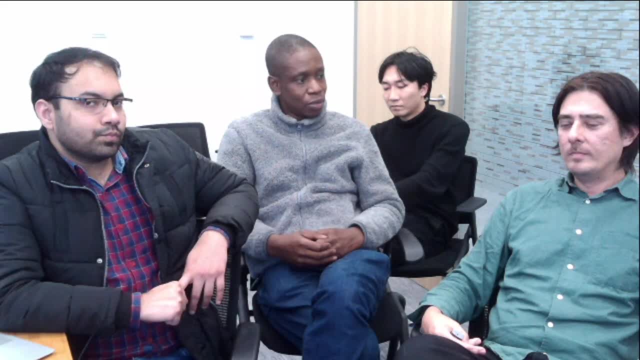 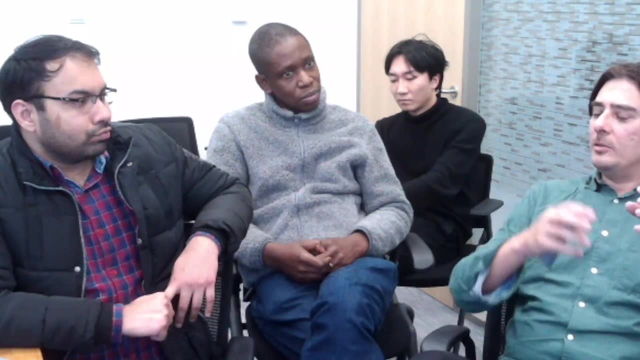 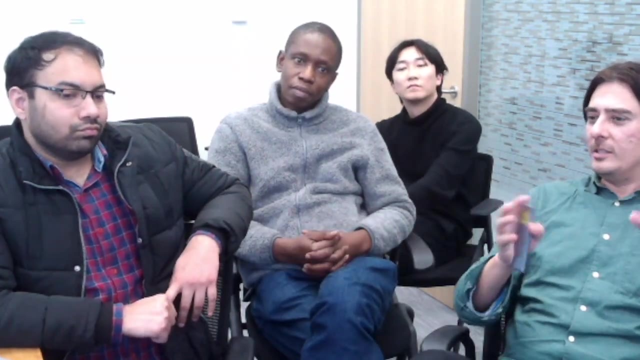 because this is showing that, maybe, far away from actually knowing or correcting errors, actually, Yeah, Well, maybe the thing here is that because the actual measurement that you need to do is quite complicated, right, This you know, ZZZZ, or? 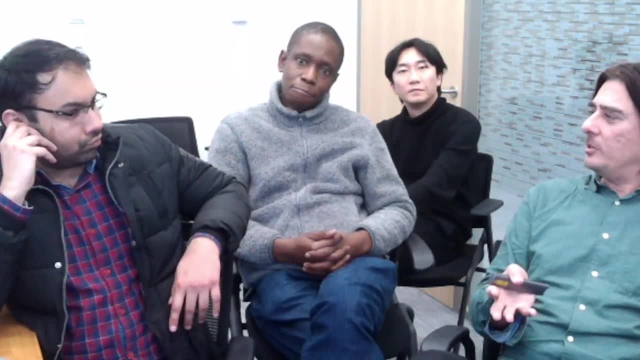 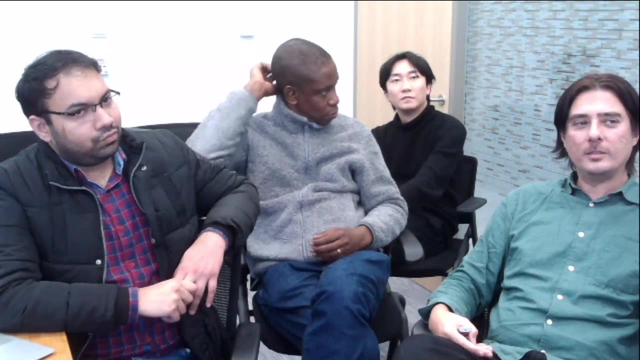 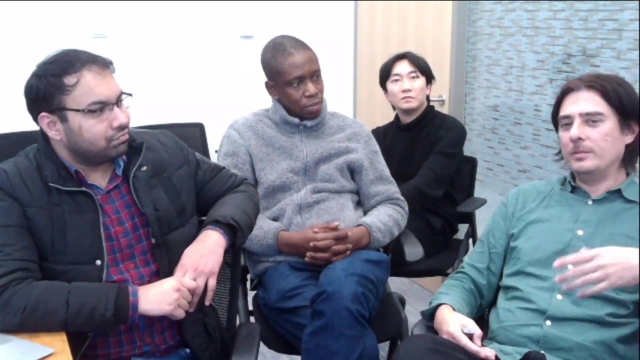 you know XXXX is a pretty complicated thing that you need to actually measure and because of that overhead, you know that introduces opportunity for more errors. right, It's not a relatively simple measurement but you know it still does it. but 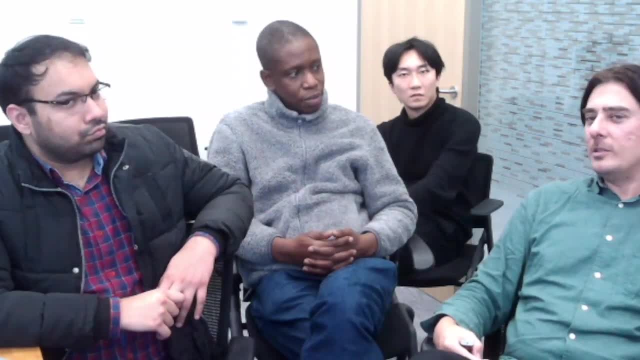 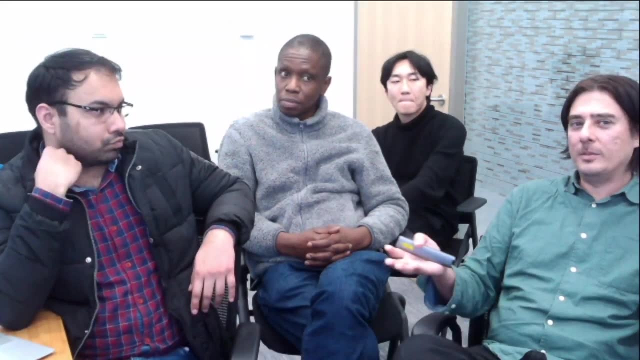 you know, I guess people have investigated quantum error correcting codes for a long time and apparently there is no simple, real simple way to do it. It's always something a bit complicated like this. I mean, surface codes are basically supposed to be the best. 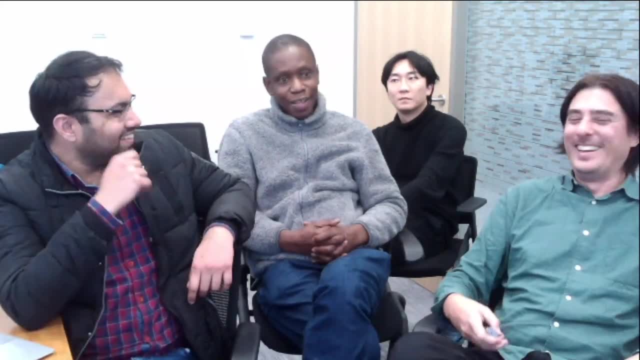 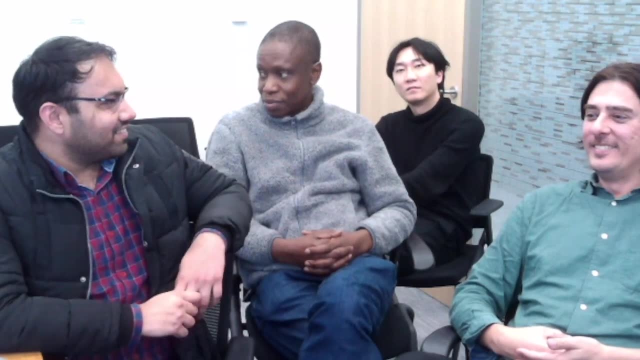 Yeah, They're supposed to be the best there is, right, All right, so you don't seem very impressed. Well, I don't know Even this idea that you know, if you scale, the larger you scale, the better. 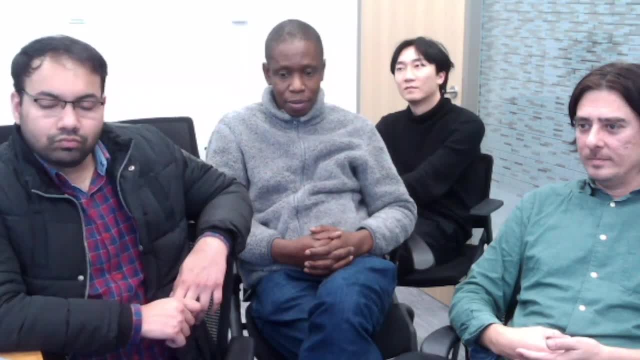 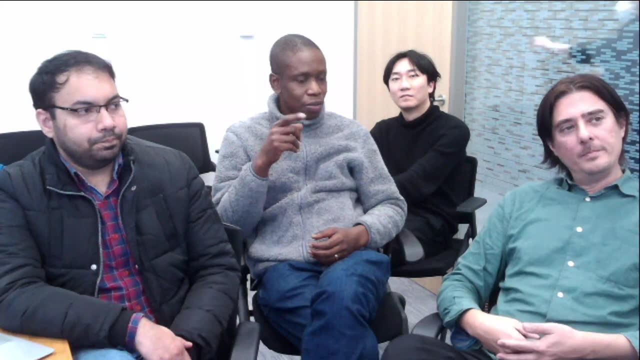 you know you're going to beat the small size thing, Okay, But if scaling bigger means more measurements and things like that, then so here they're using 25, right, Yep, So assuming they're able to.